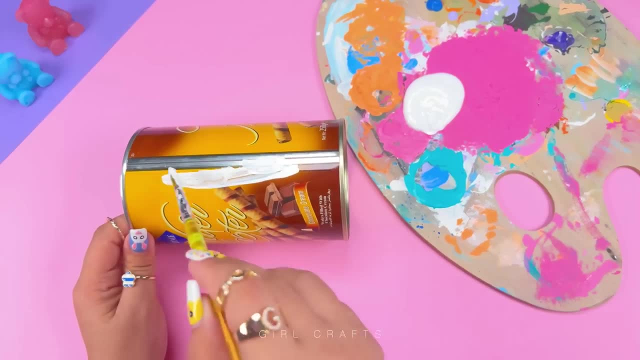 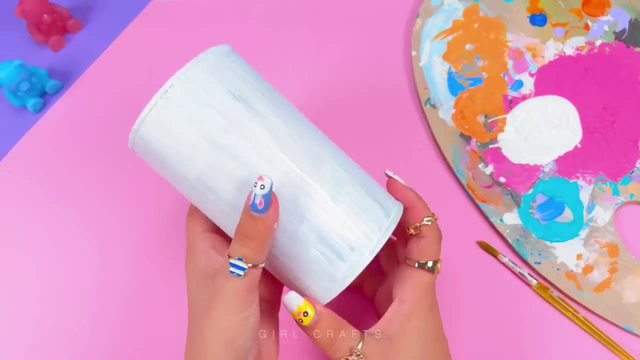 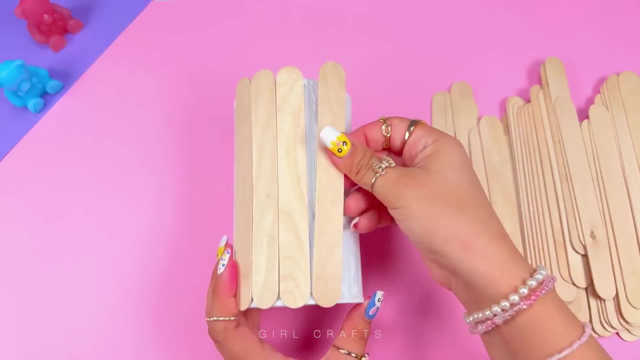 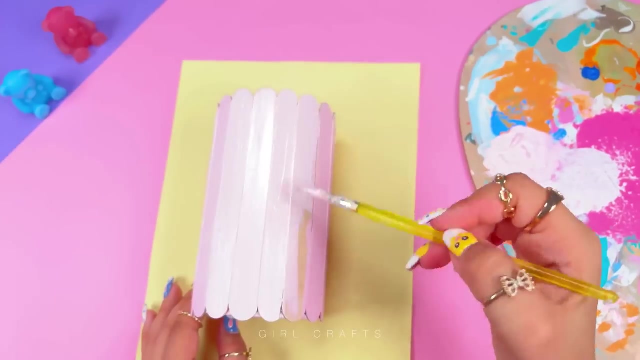 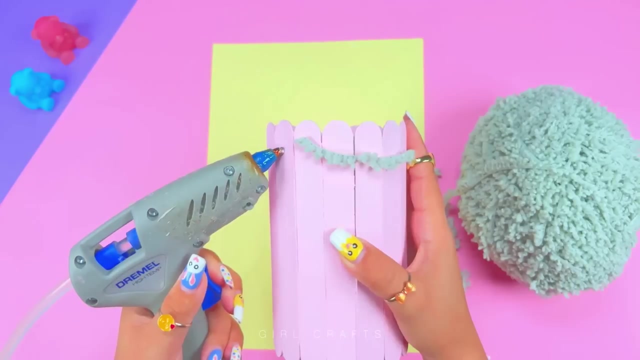 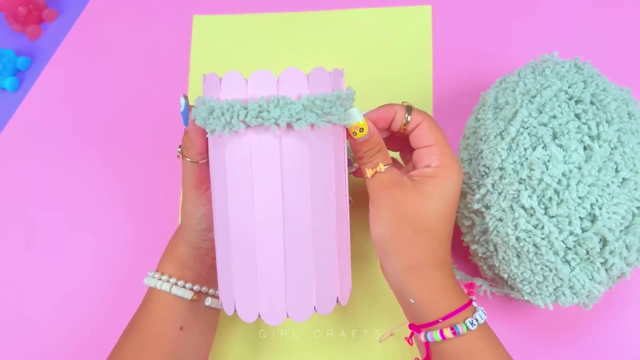 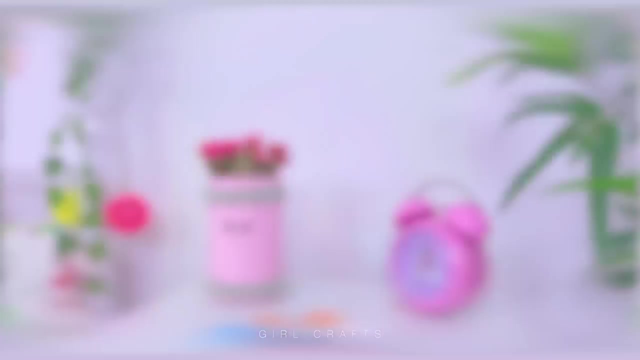 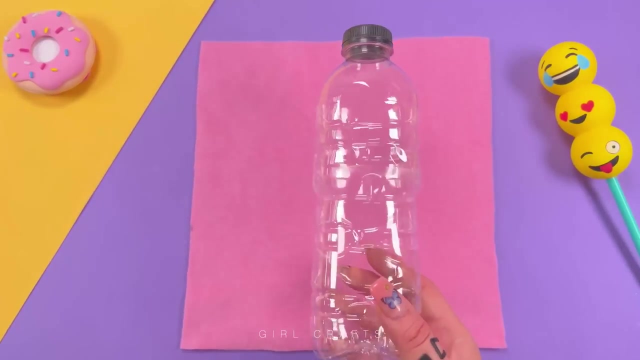 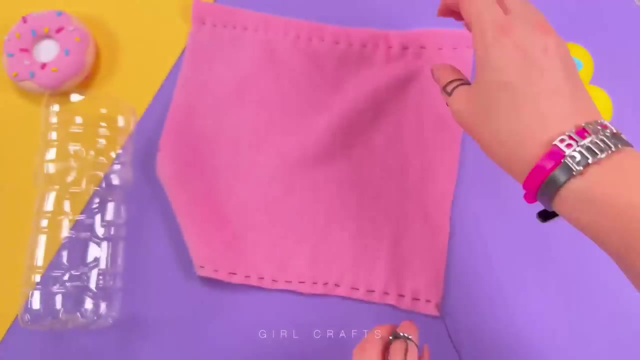 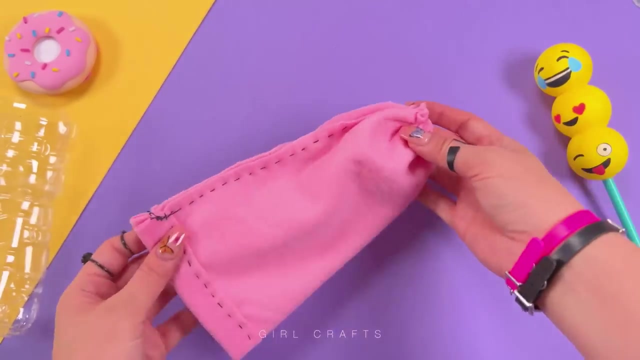 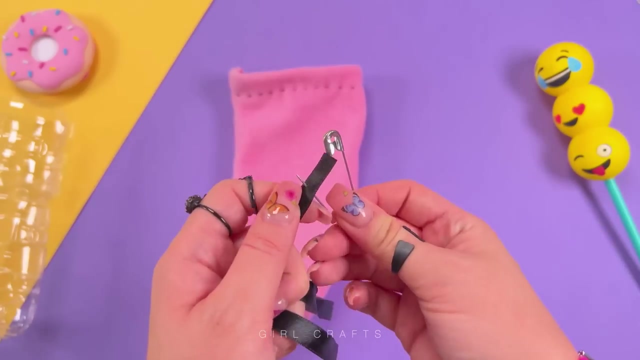 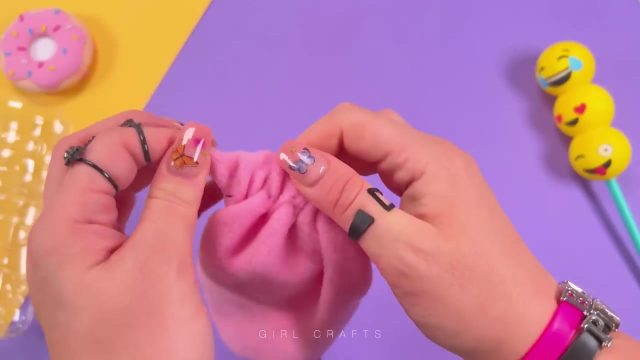 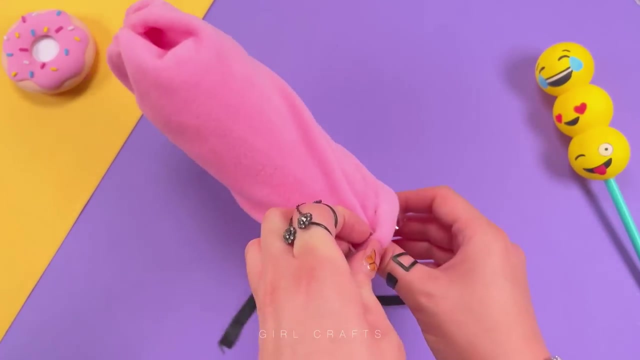 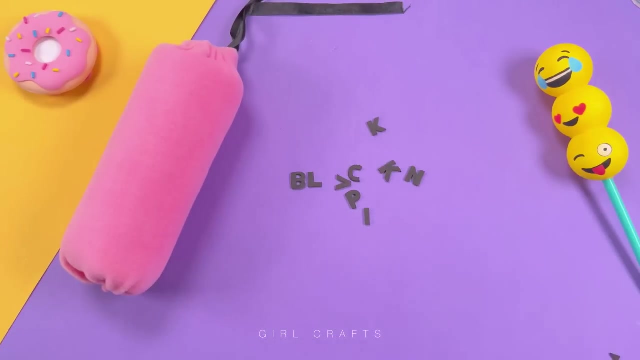 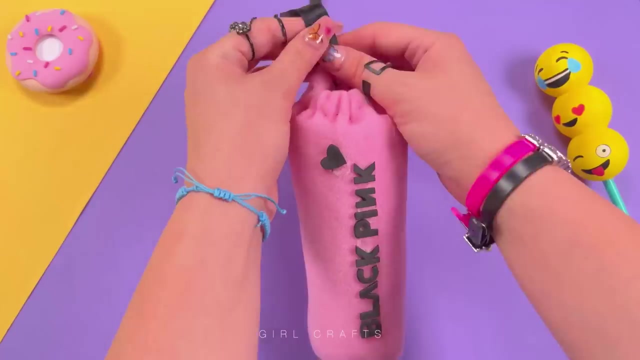 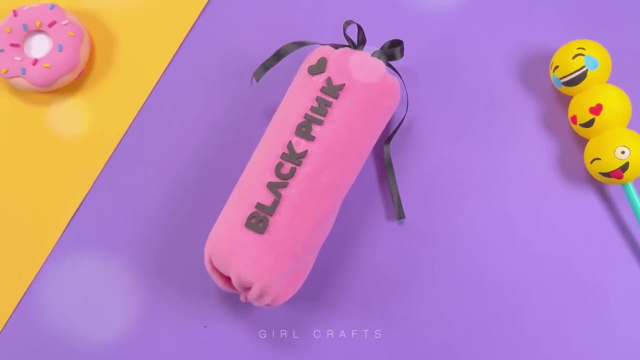 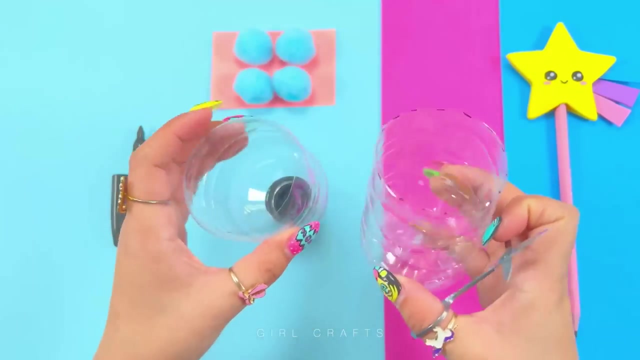 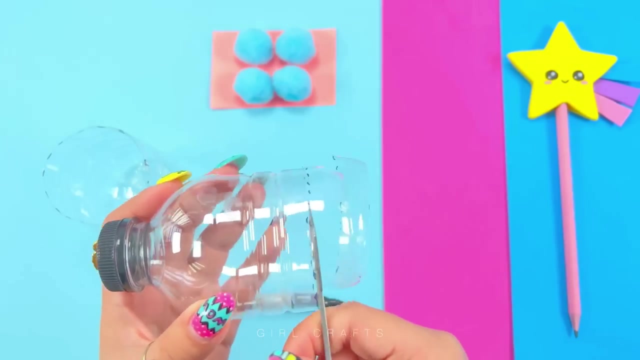 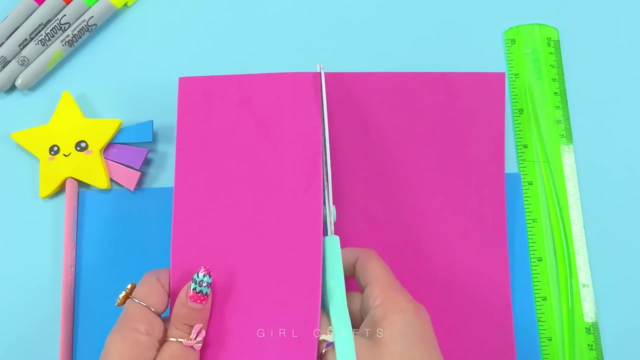 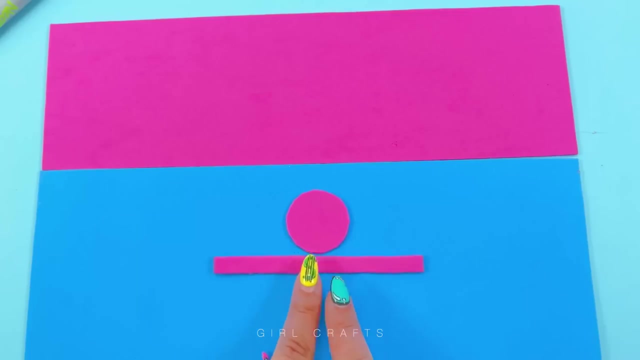 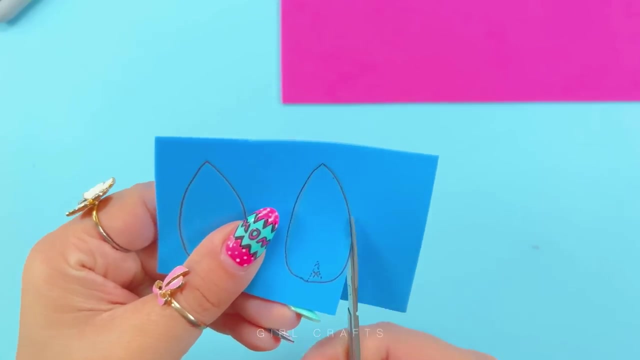 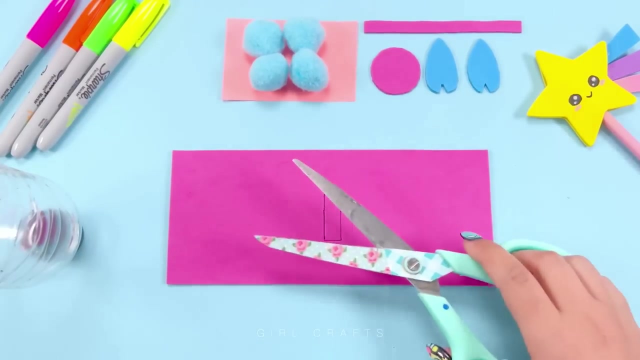 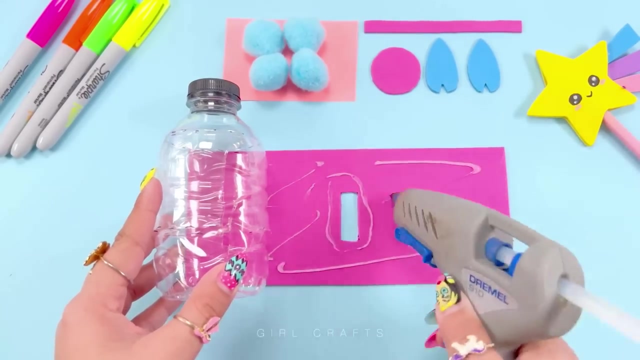 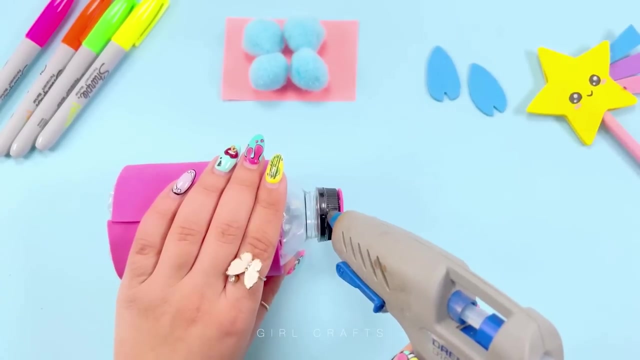 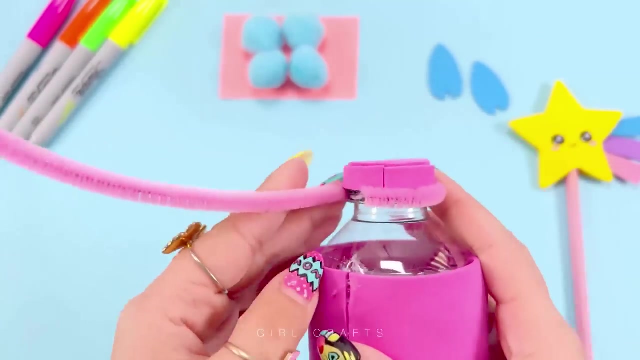 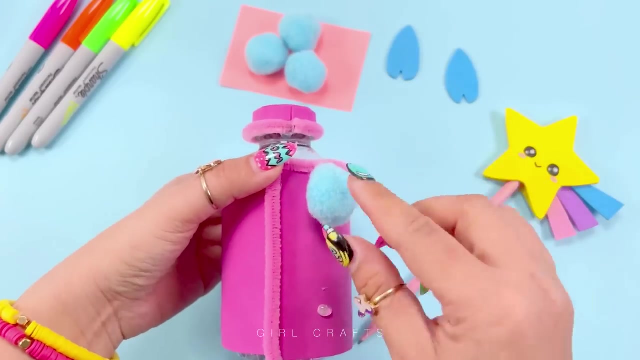 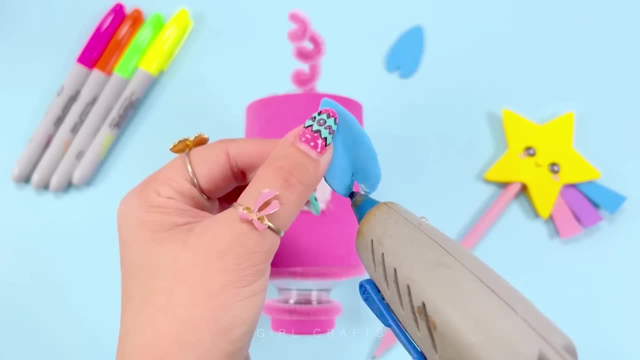 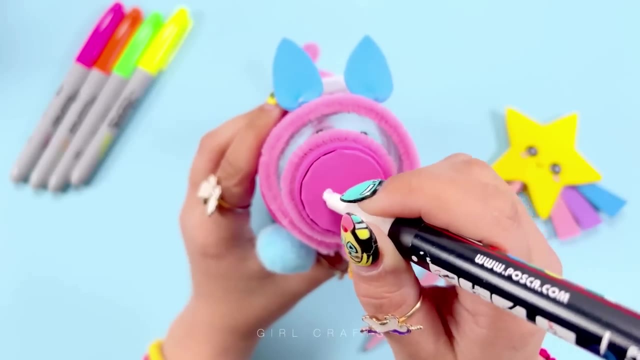 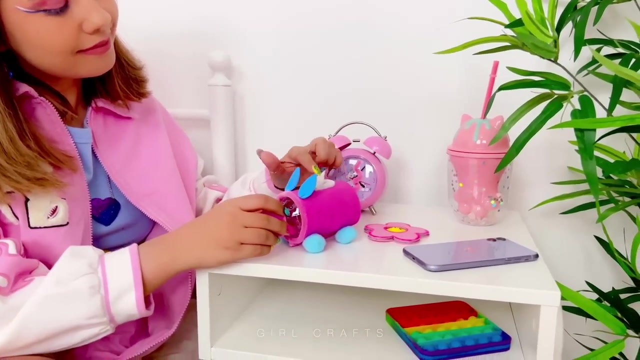 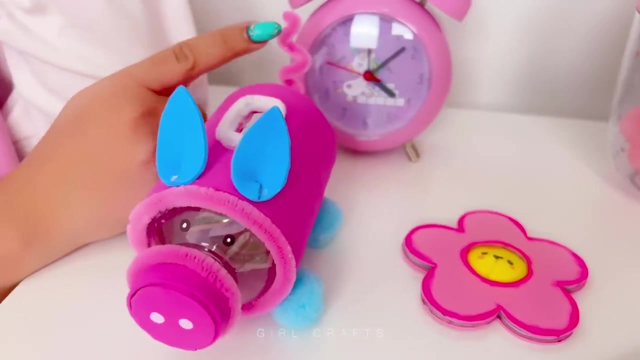 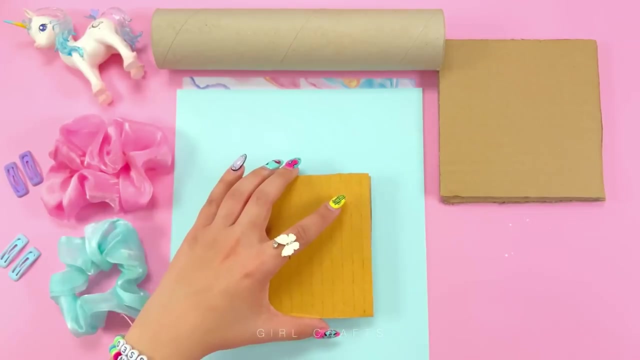 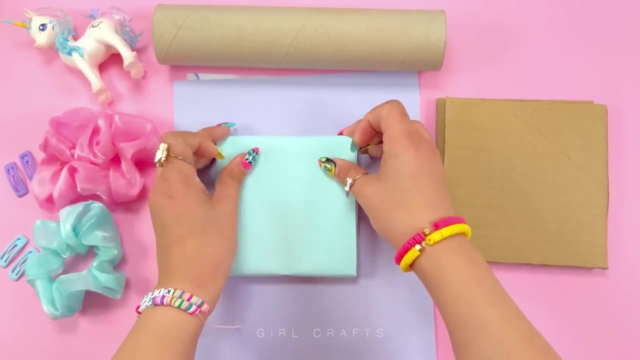 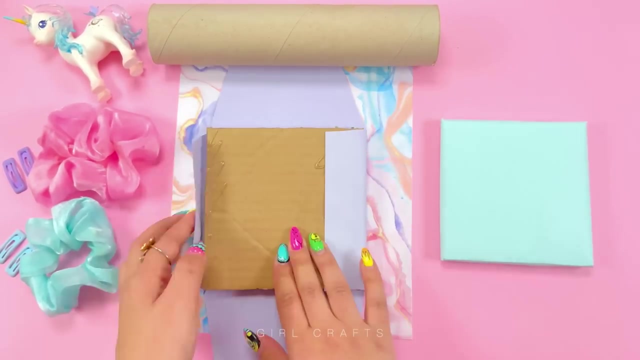 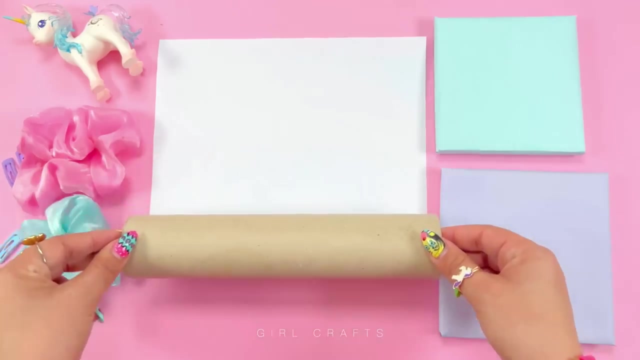 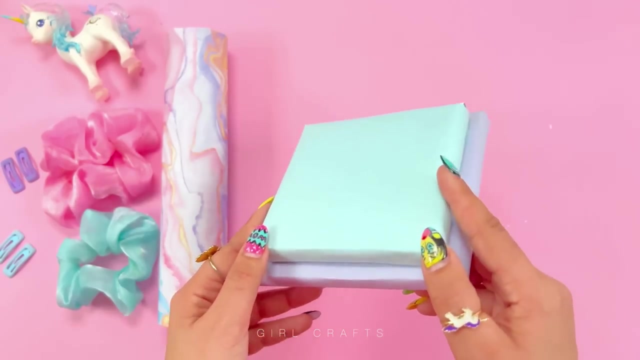 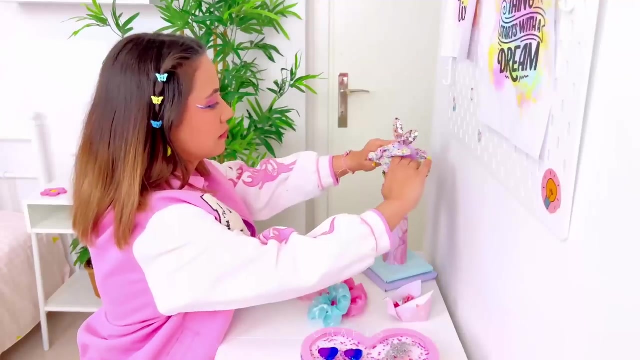 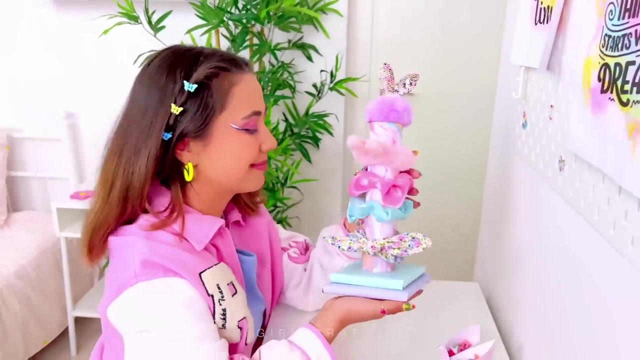 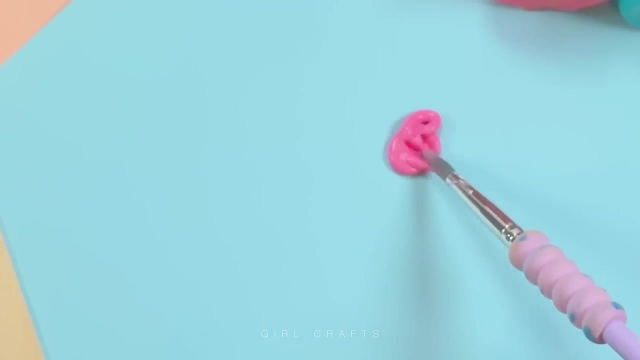 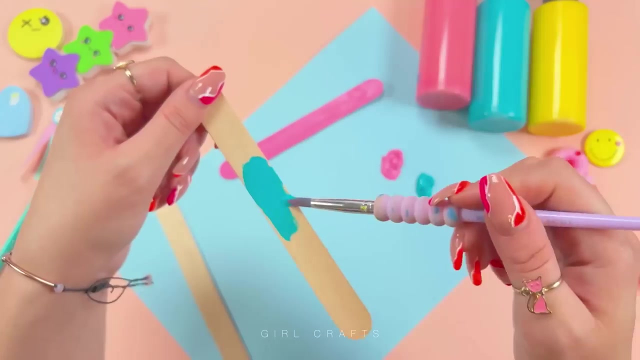 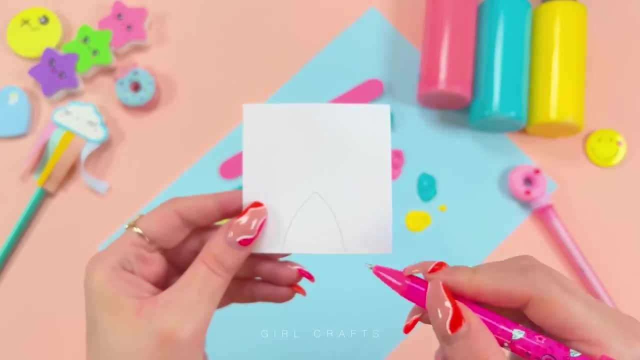 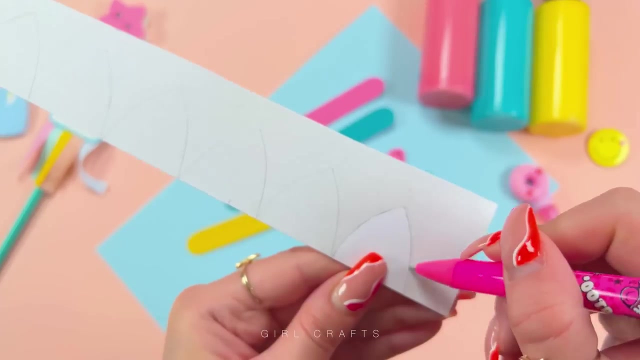 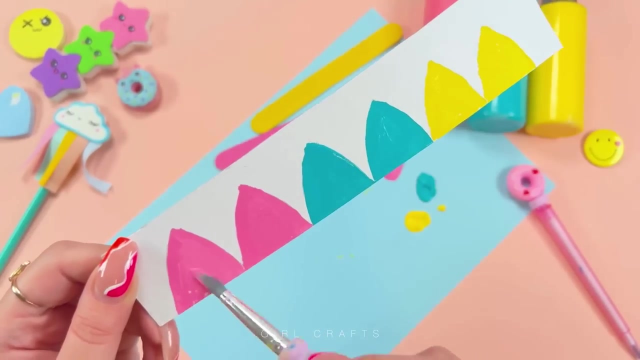 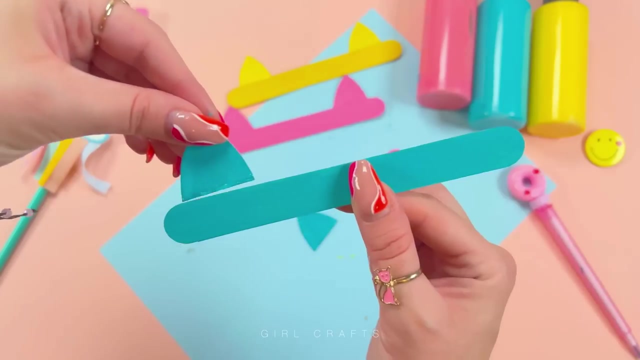 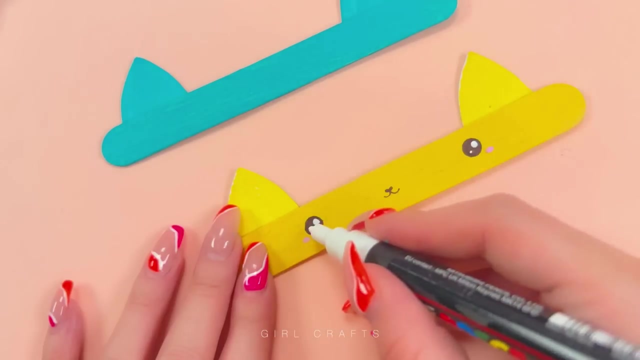 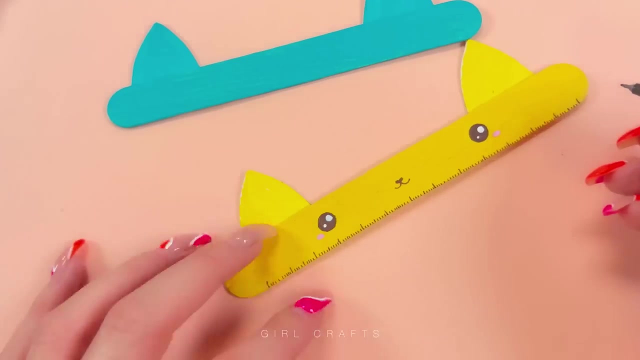 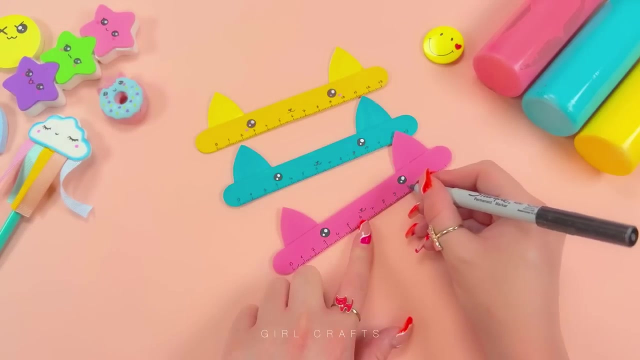 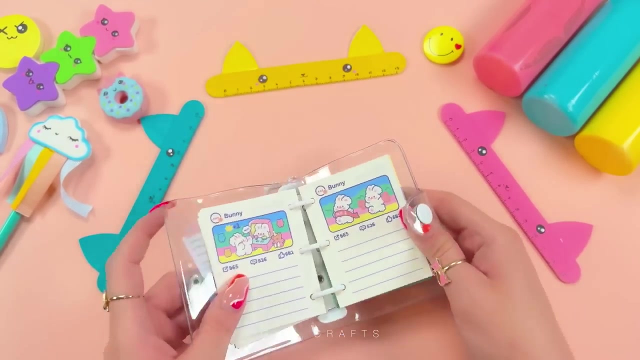 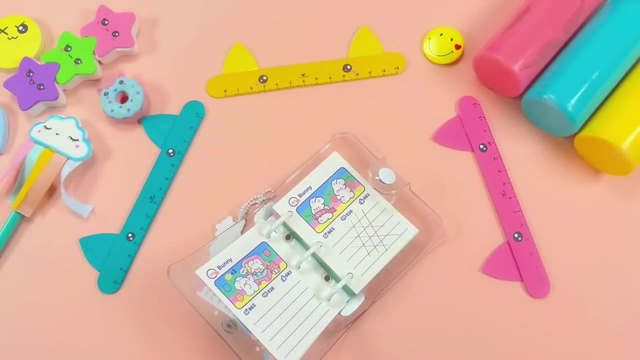 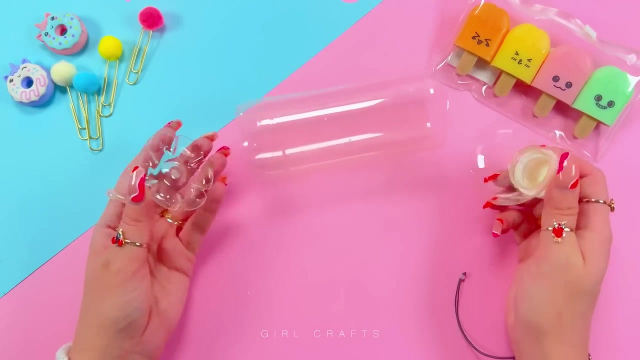 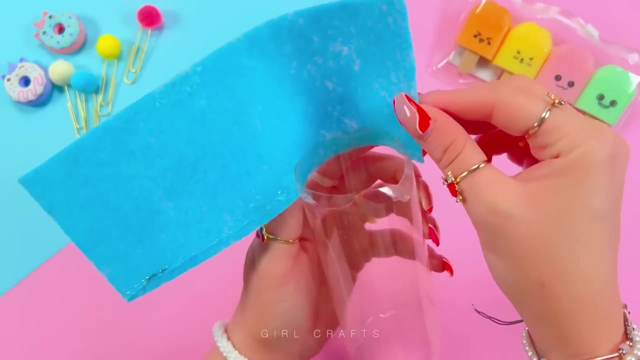 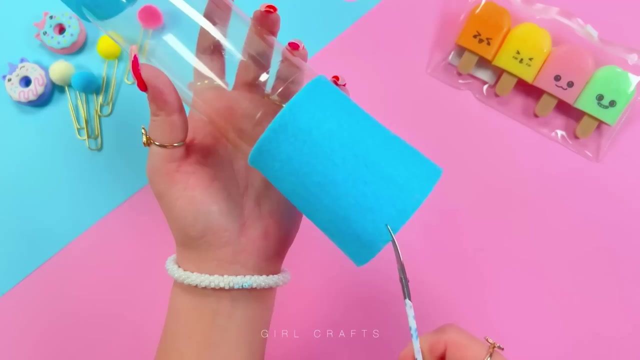 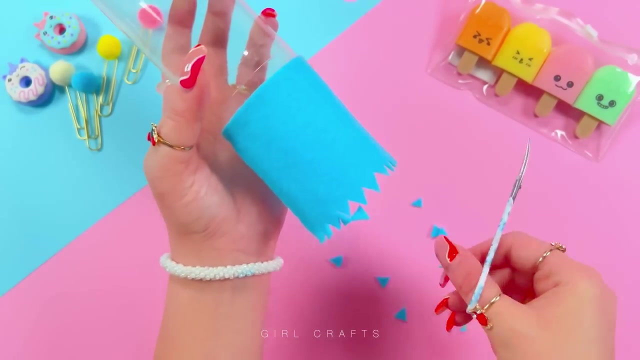 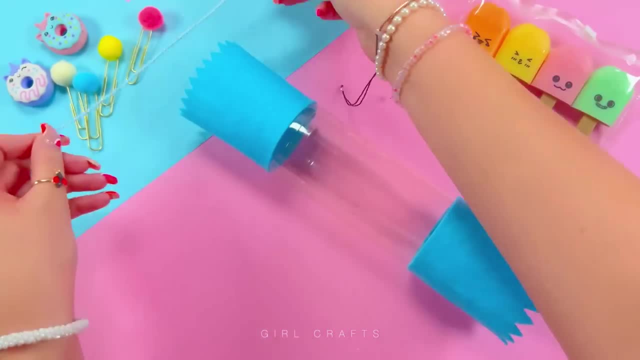 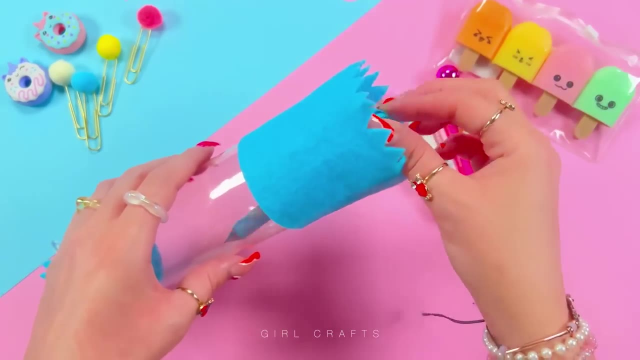 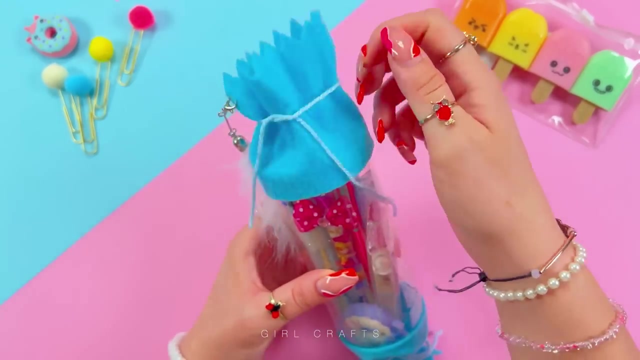 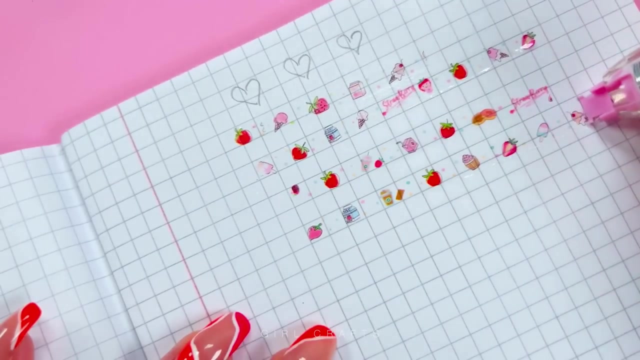 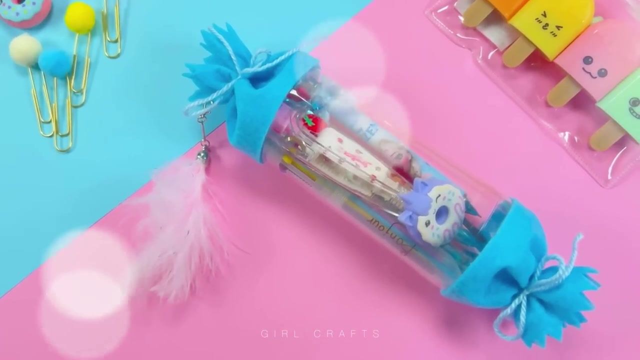 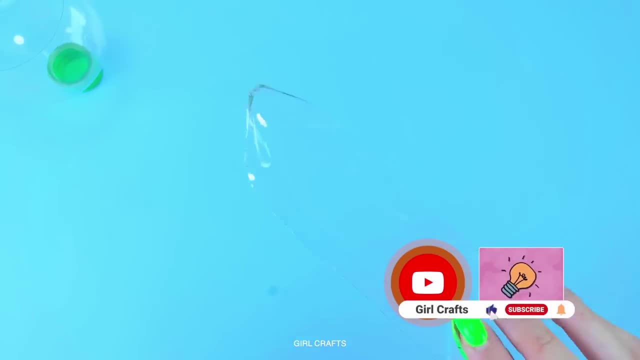 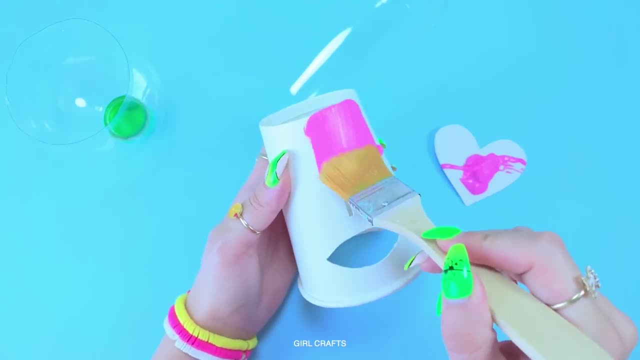 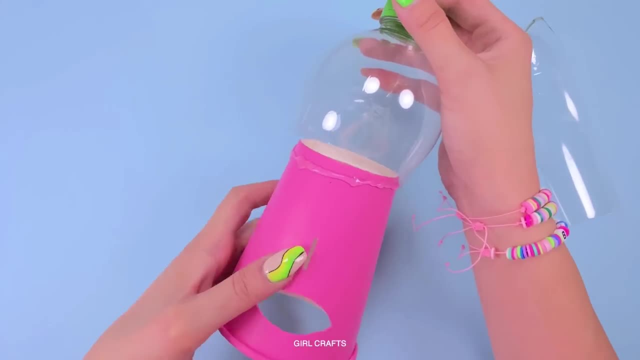 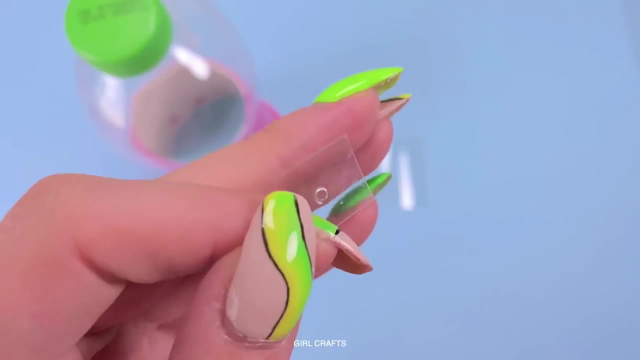 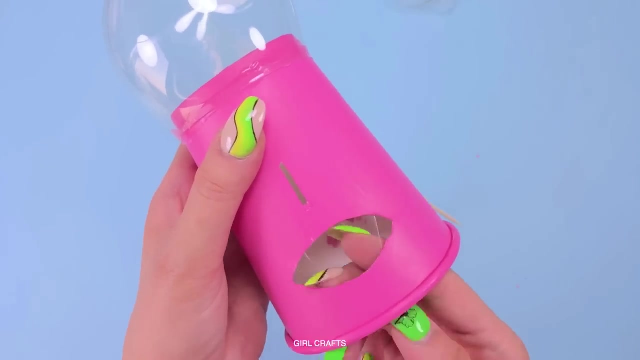 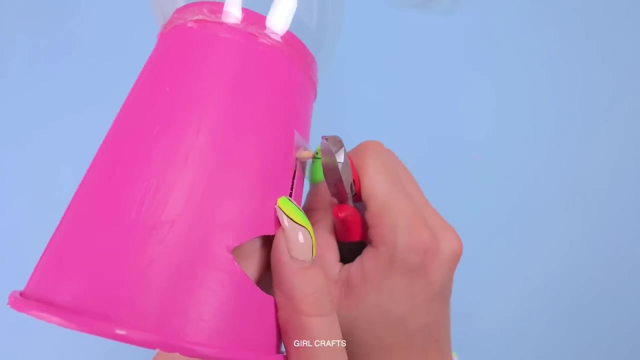 We hope you enjoy the drive. Shine like a star cause. you know that you are Free. mind every kind. I just came to have a good time. Now everybody here's fine, Feels good on cloud nine: Yeah, everything is here right here, right now. 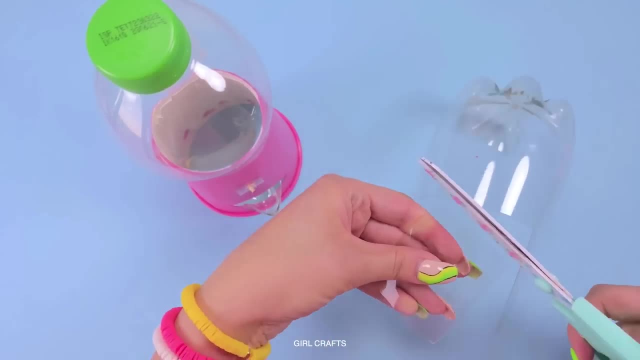 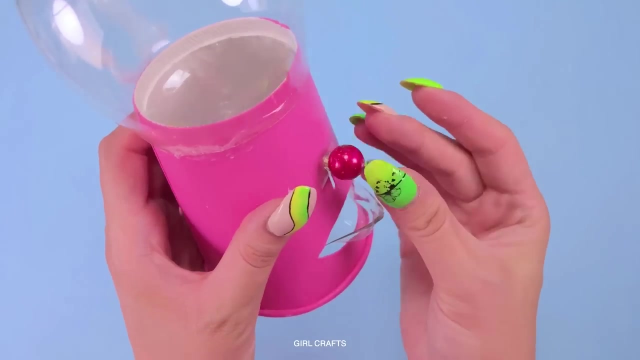 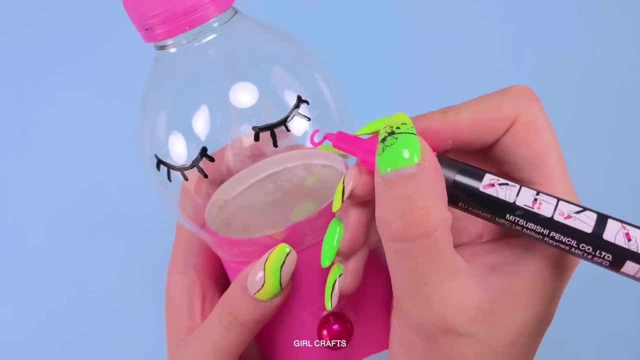 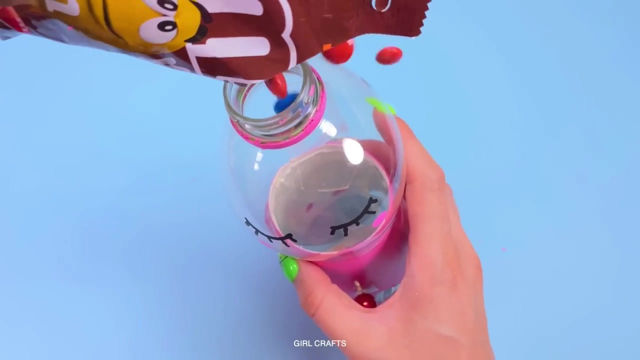 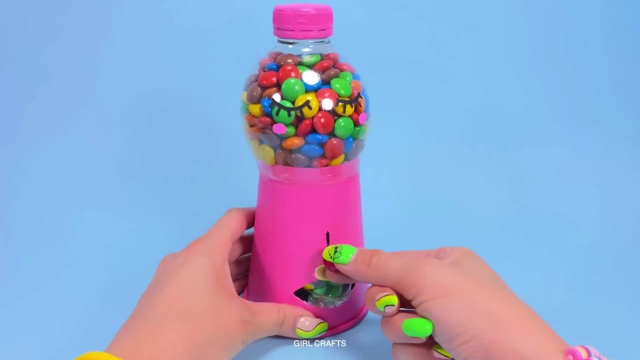 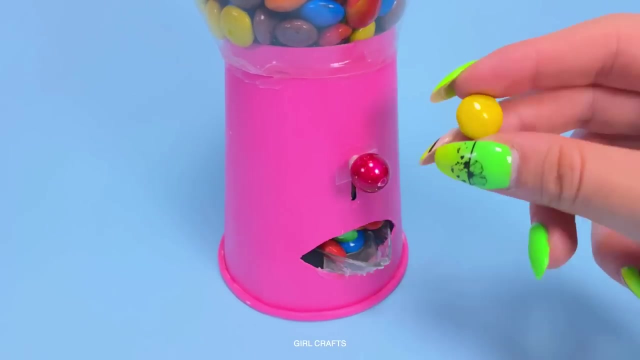 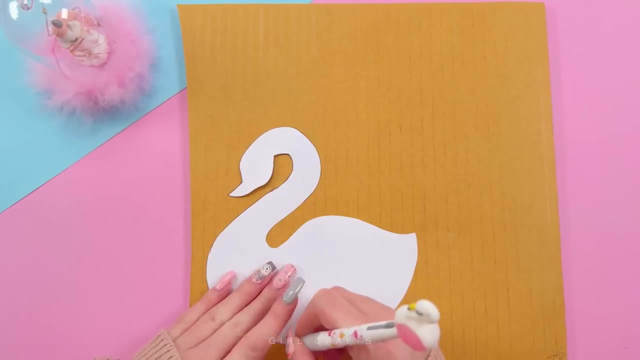 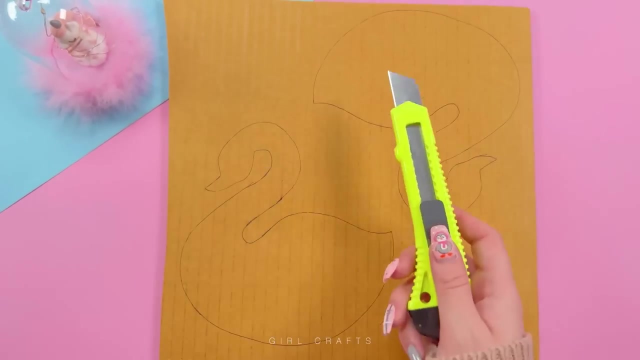 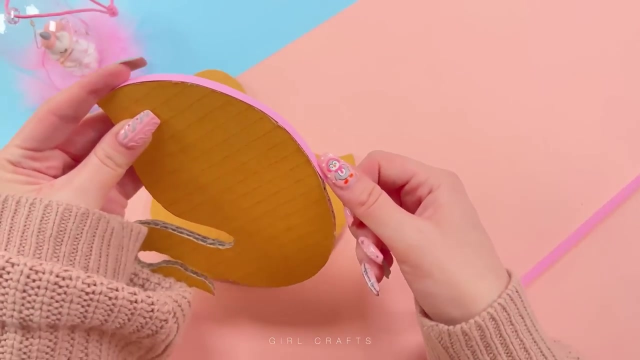 So here I am, one of a kind And bottom line. I'll draw my own design. I'm reaching for The diamond skies. Make you whistle like When I drive by. I say, hey, Shine like a star cause. you know that you are. Star comes through Free mind every kind. 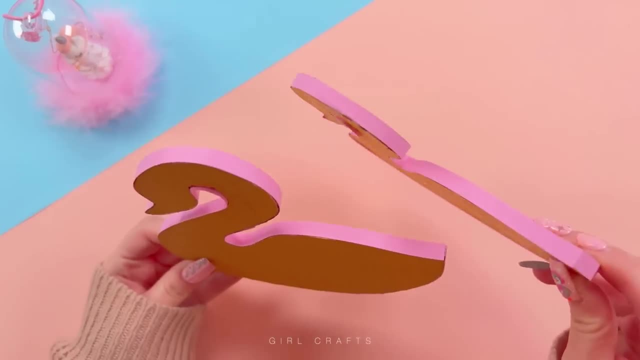 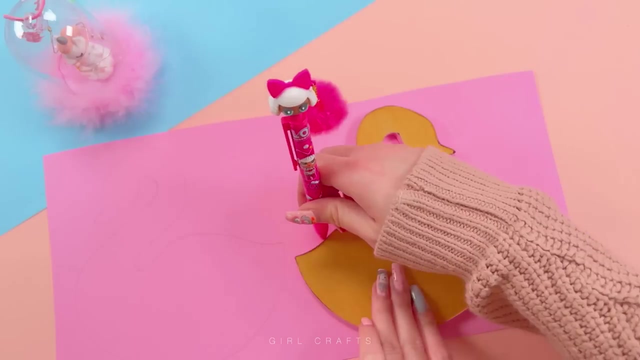 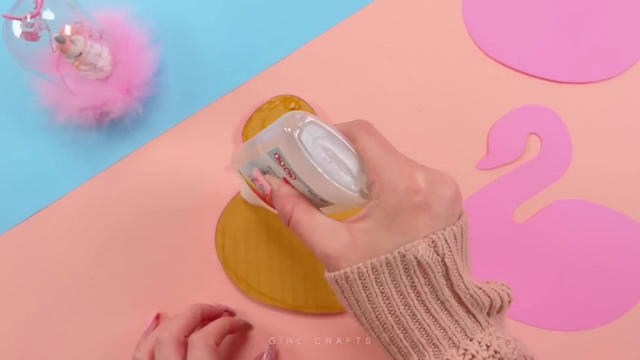 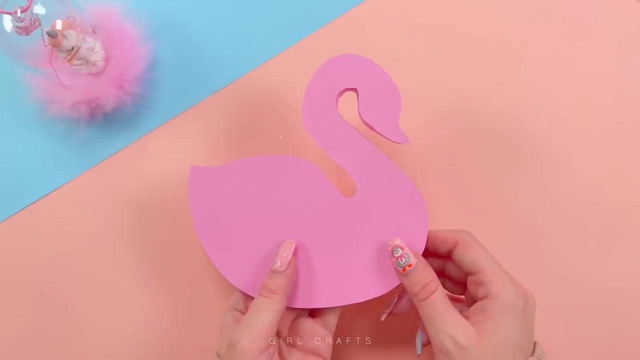 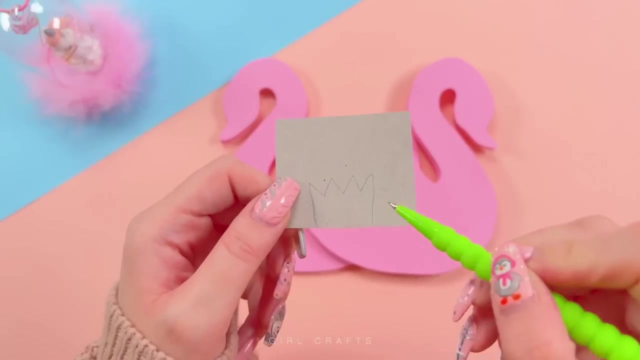 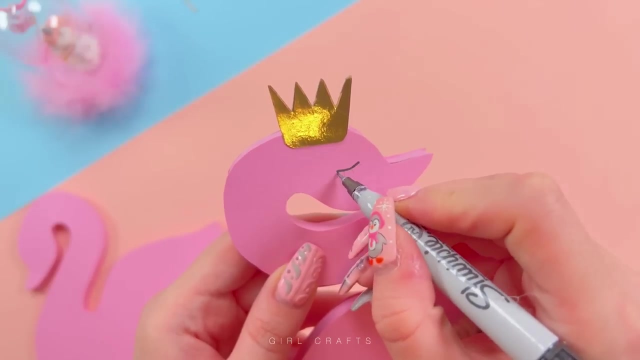 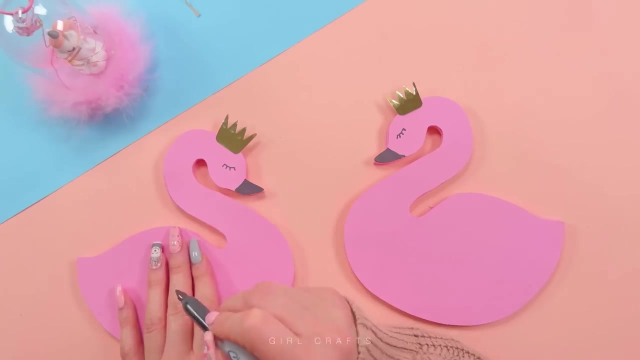 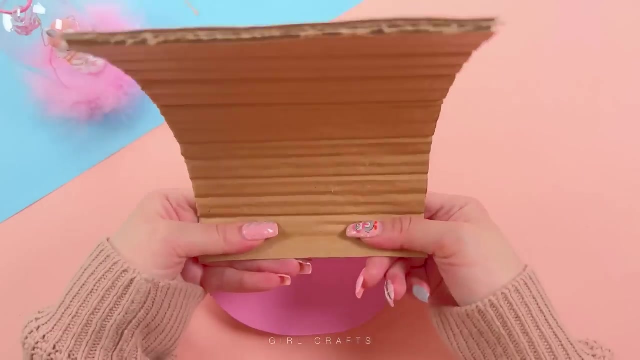 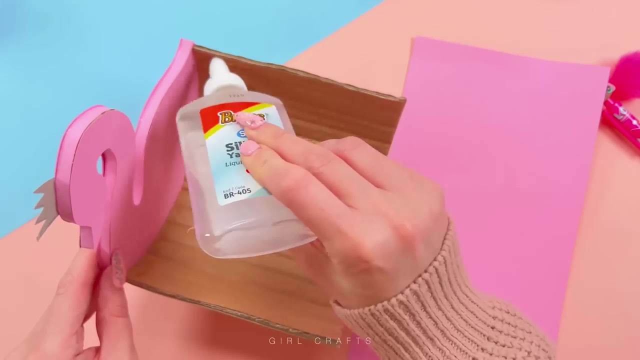 I just came to have a good time Now. everybody here's fine, Feels good on cloud nine. Yeah, everything is here, right here, right now. I just came to have a good time Now, everybody here's fine, Feels good on cloud nine. Yeah, everything is here, right here, right now. Oh, oh, oh, oh, oh, oh, oh. I'll get out again. I'll get out again. I'll get out again. It's been a while since we felt the way we did Back when we were dumb and younger. It's been a while since I looked into your eyes. 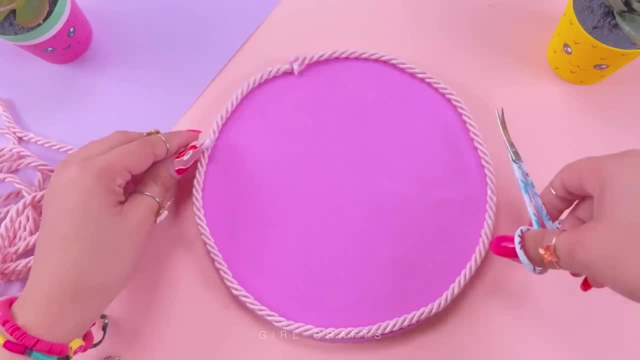 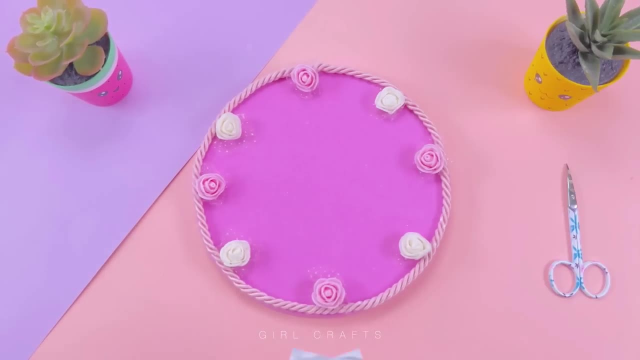 And saw starlight, bold, bright colors. yeah, When I'm down, when I'm dry, When I'm down, when I'm dry, When I'm down, when I'm dry, When I come, no one else Put my love, my love. 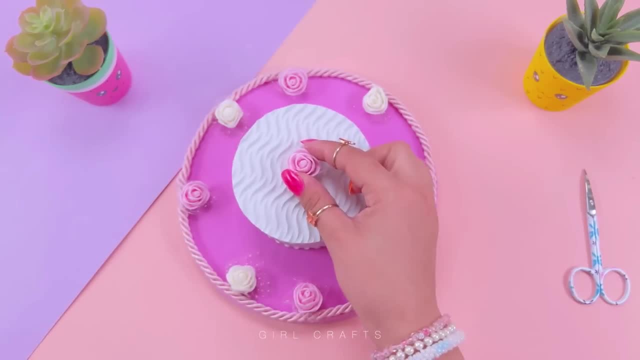 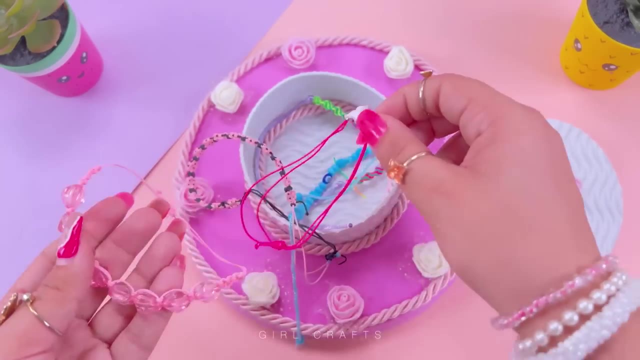 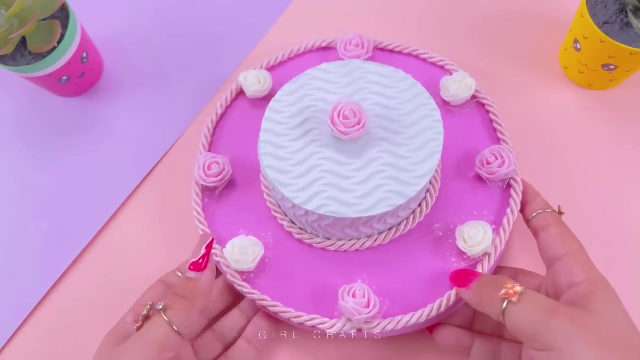 I would choose you over and over. I would choose you over and over. I would choose you over and over again again. And the past are all we've been through. There's no one else for me but you. I would choose you over and over, again, again. 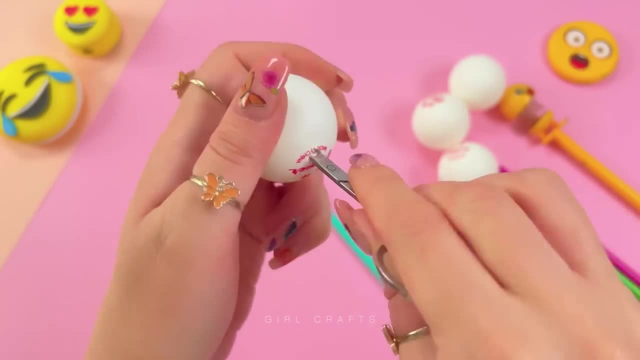 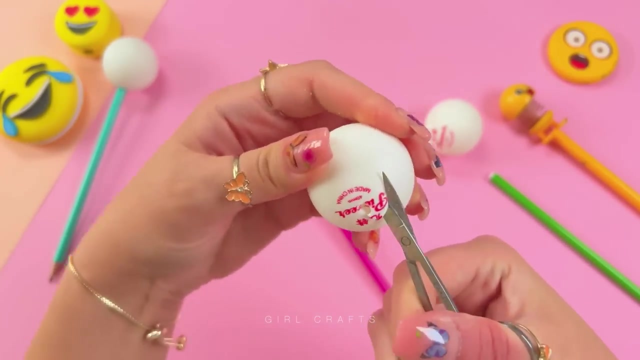 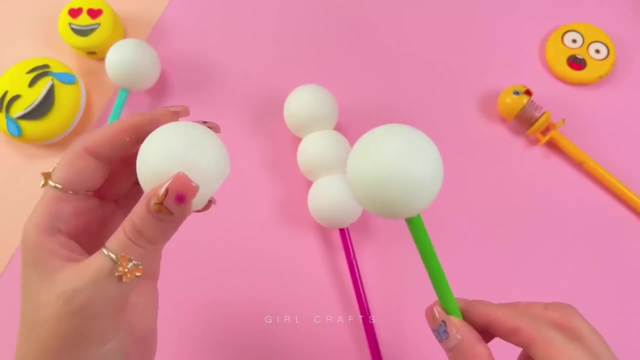 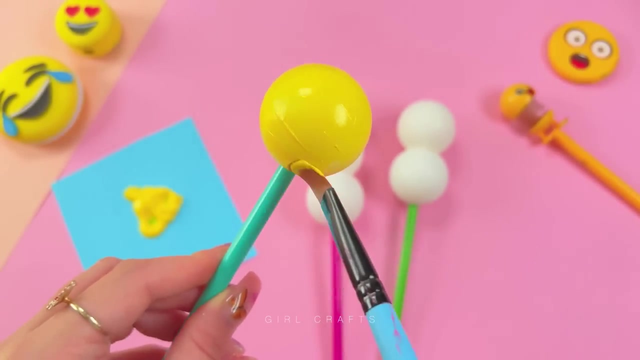 I'll get out again And you are the real thing, The novel before the film, All the nuance, every letter, And you do things to me Like they have never been done. A love like ours could last forever And ever. when I'm down, When I'm down. 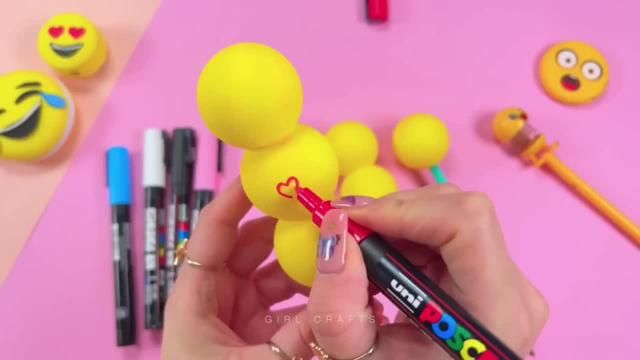 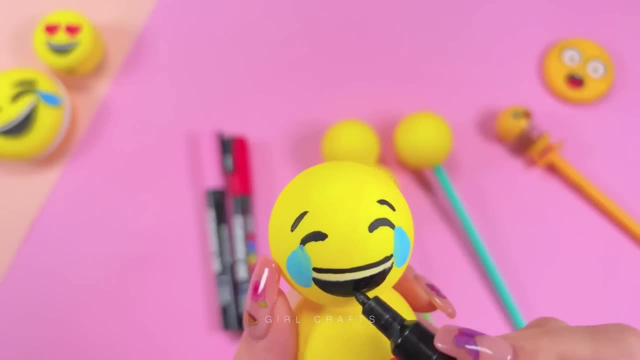 When I'm flat- Até quem me leva. When love comes through- A love like ours could last forever, And the past are all we've been through. There's no one else for me but you. And when I'm down, Oh baby, Put your money down. 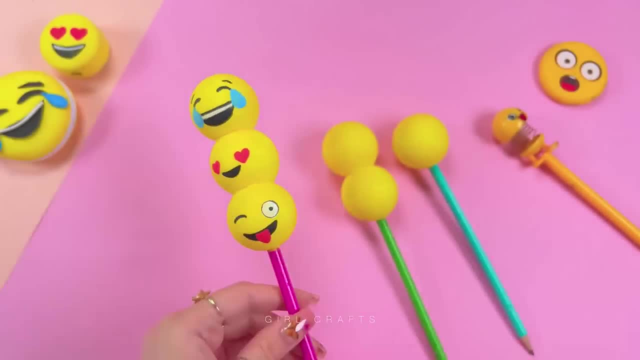 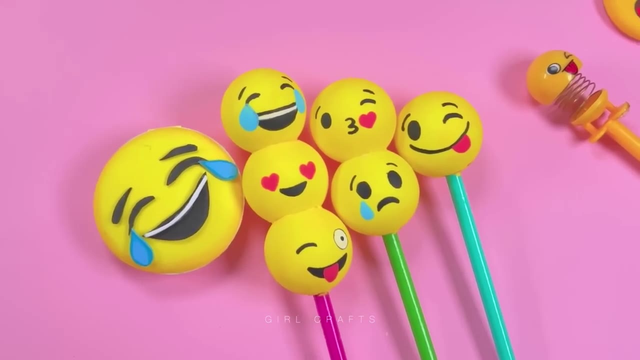 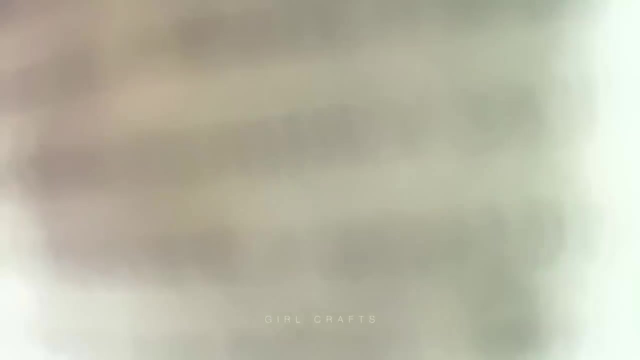 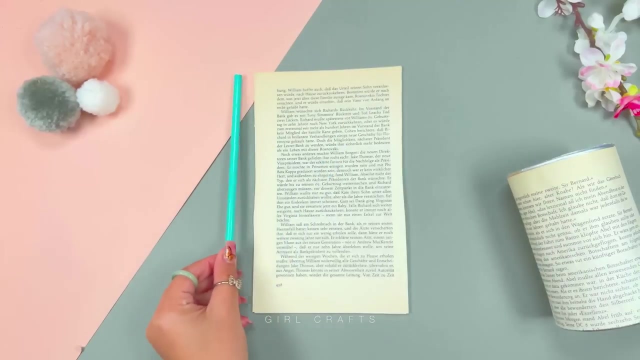 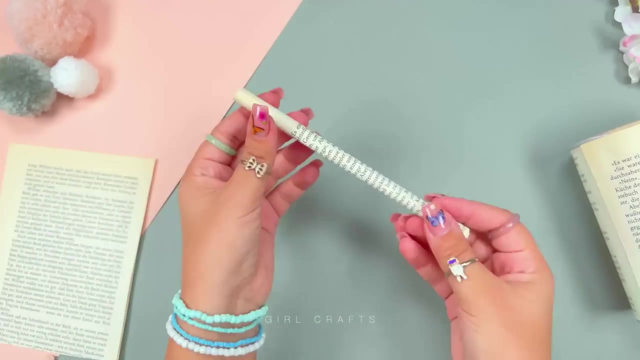 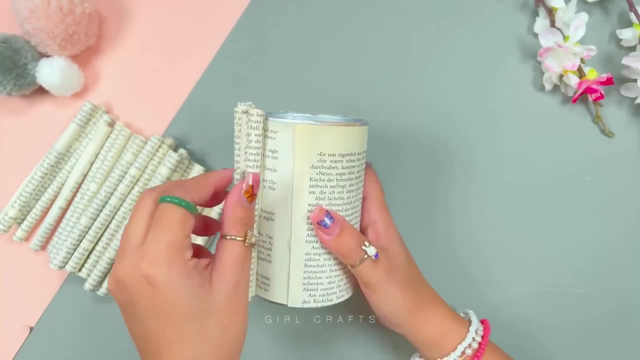 Turn you down A love like this. Every time we're in love, Every time we're having fun, Are you glad? car Every time we're in love, Is it true? When I'm down, when I'm dry, No one else, no one- My love. 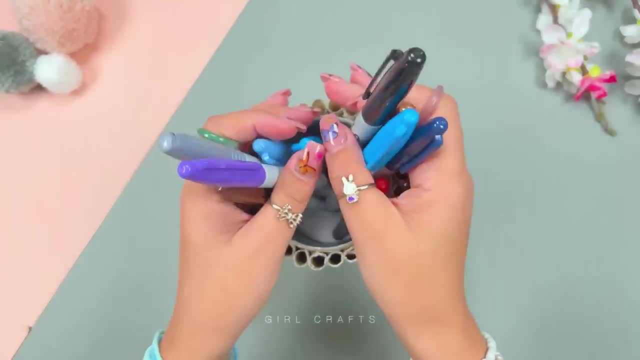 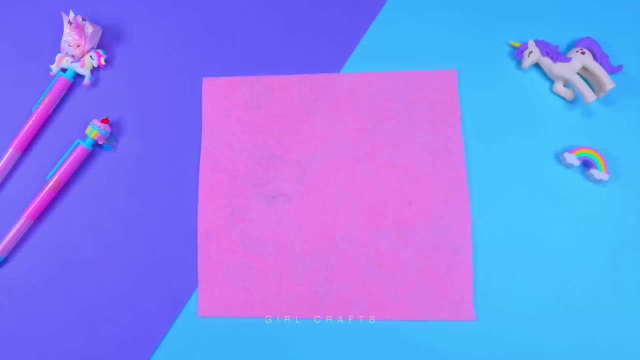 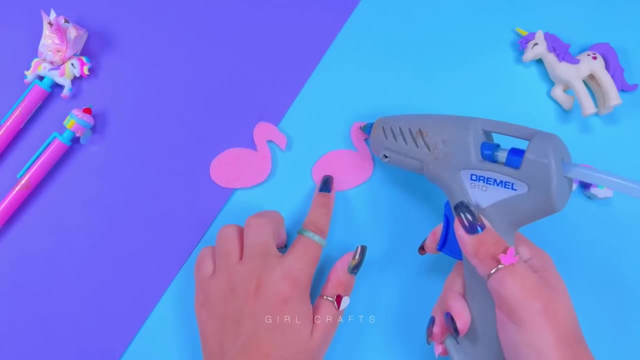 I would choose you for it all. I would choose you for it right over. I would choose you for it right over again Again. And I still hope we've been through this. No one else can be but you. I would choose you for it right over again, Again. 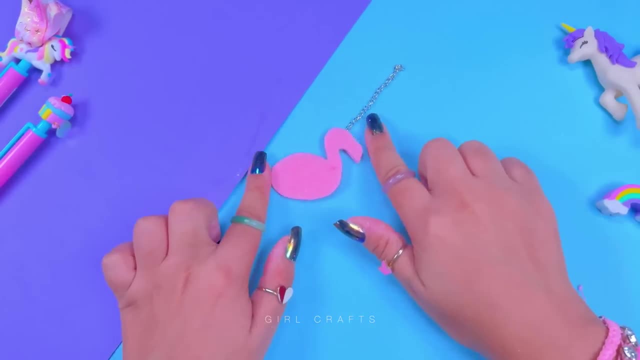 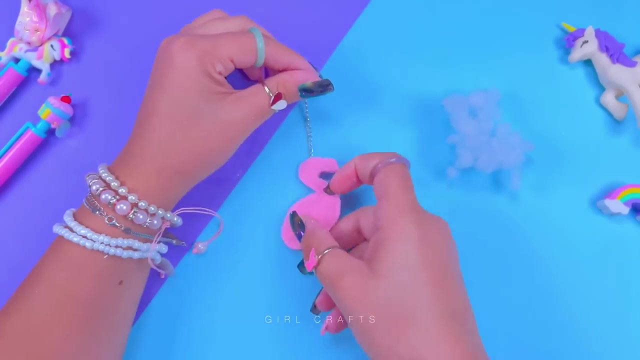 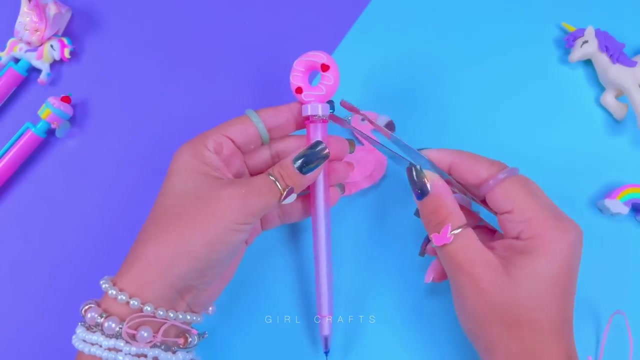 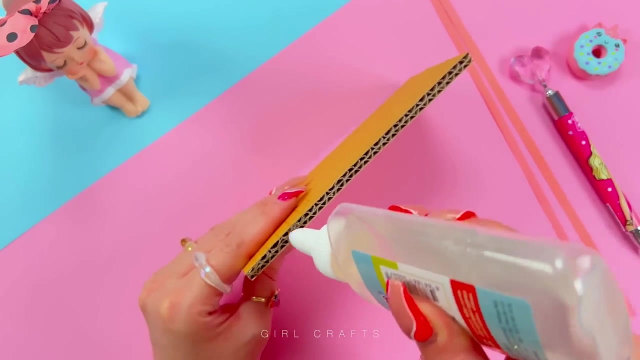 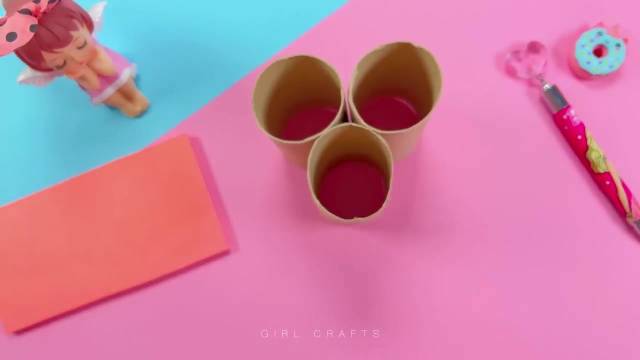 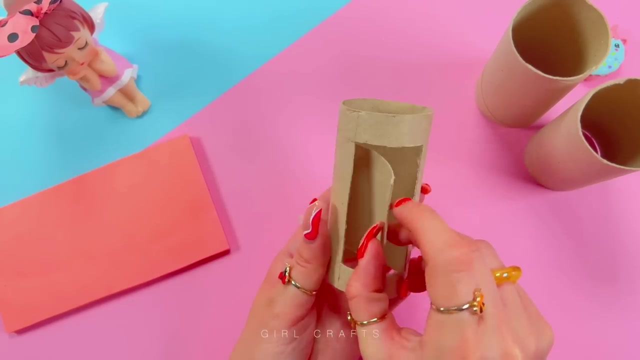 I would choose you for it right over again Again. I would choose you for it right over again Again. Can you tell me why you hang up, Or maybe what I need to do To keep you on the phone, So we can think this through, And I just wanna talk to you. 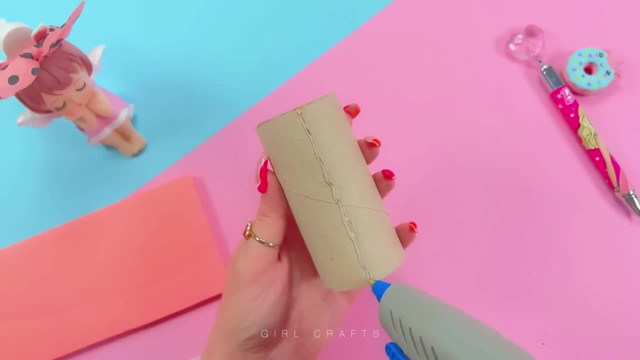 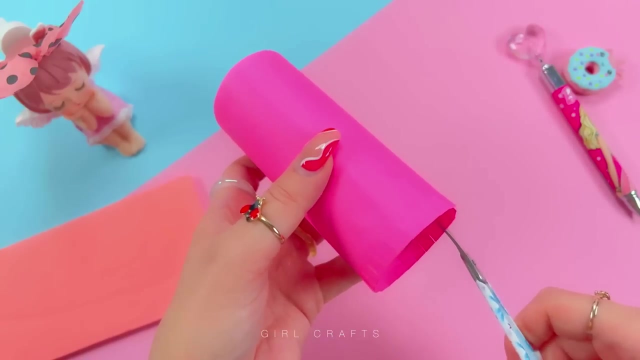 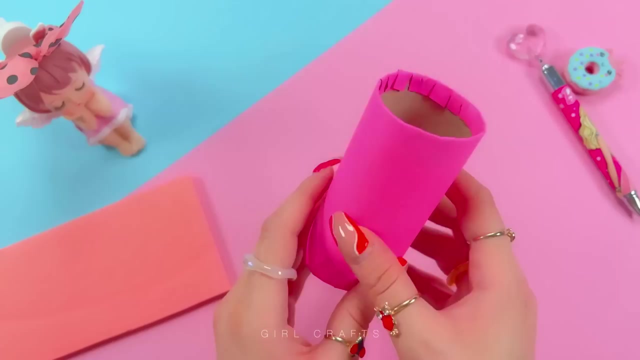 And give you every single reason why. But I can't get through. I can't get through to you, And the hardest part is waiting on the sun to come. So when you lay awake in bed tonight, I hope you think of all the times You left the conversation. Waiting for a chance. You never came in. Now you'll never get to see All the possibilities. Could have happened all tonight. But no, We'll wait till tomorrow, Maybe when you wake up. Oh, You think that you can call me back, So we can work this out. So we can work this out. 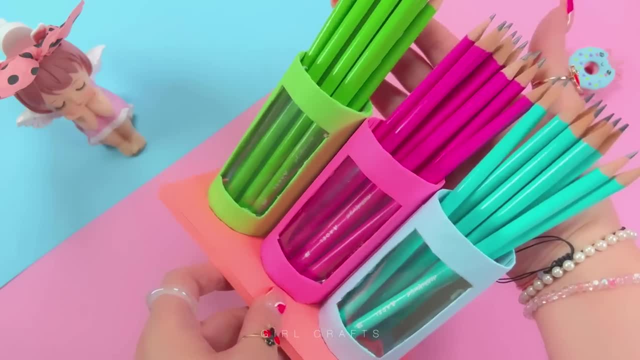 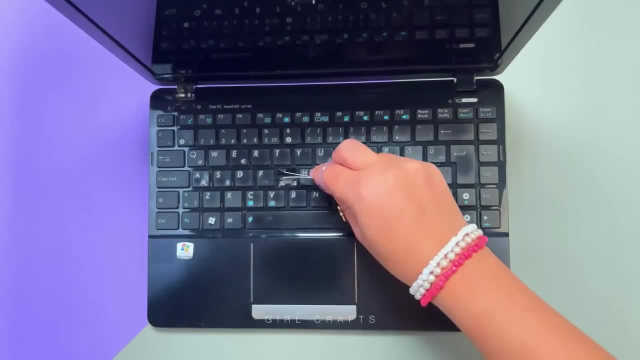 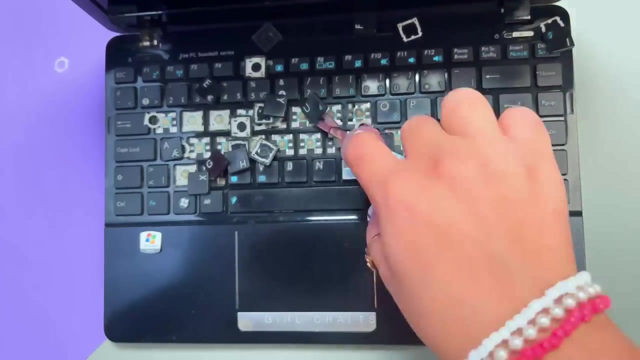 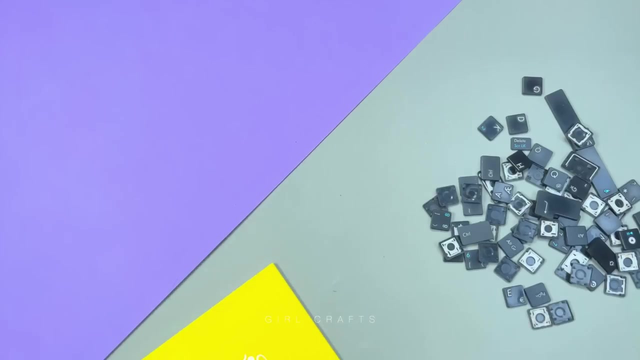 And now that you're relaxed, Focus on the details. Come on, Remember why we fell in love, Let's think about the good stuff, Let's think about what makes us, And the hardest part is waiting on the sun to come. So when you lay awake in bed tonight, 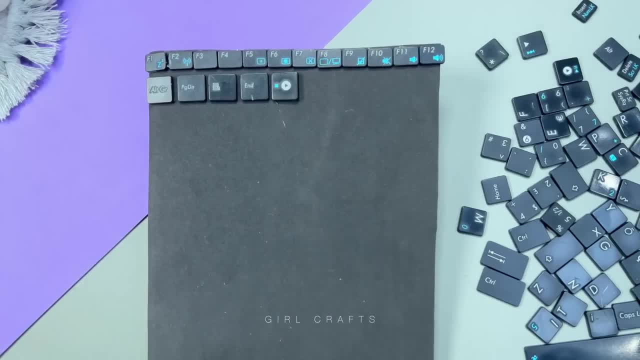 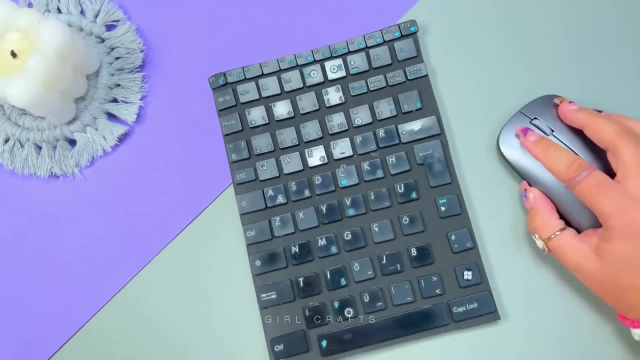 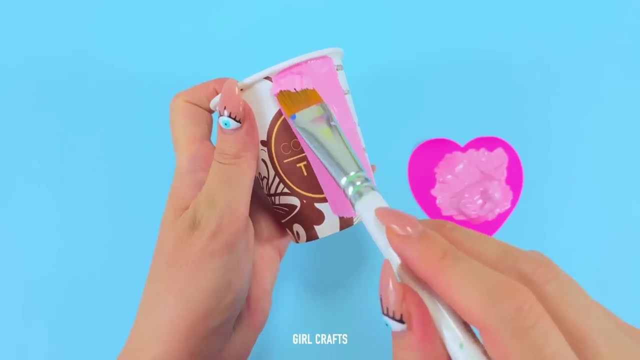 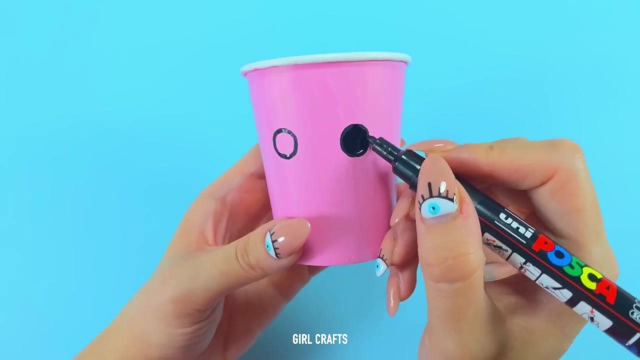 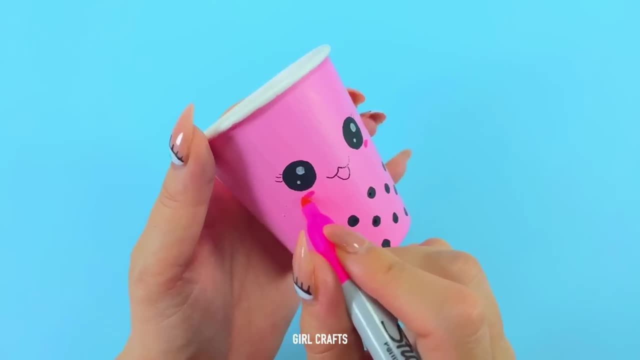 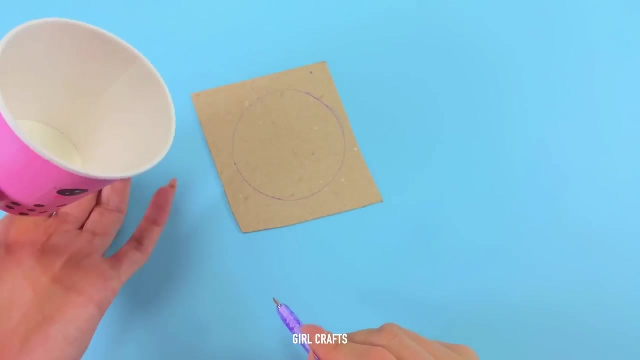 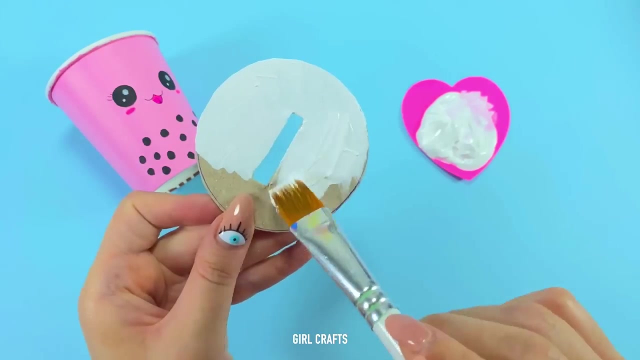 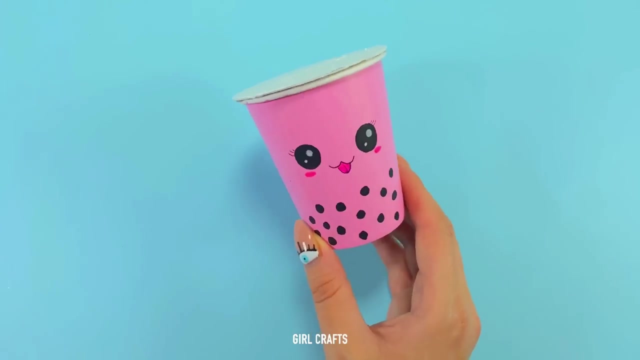 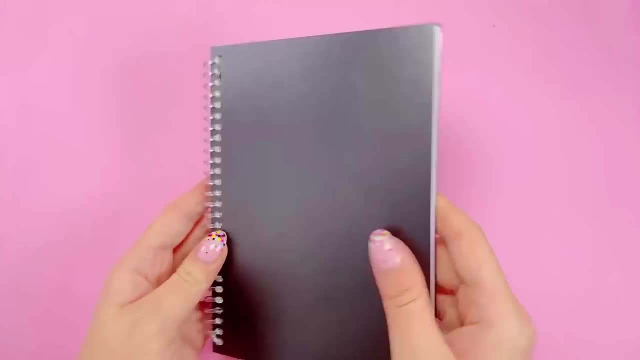 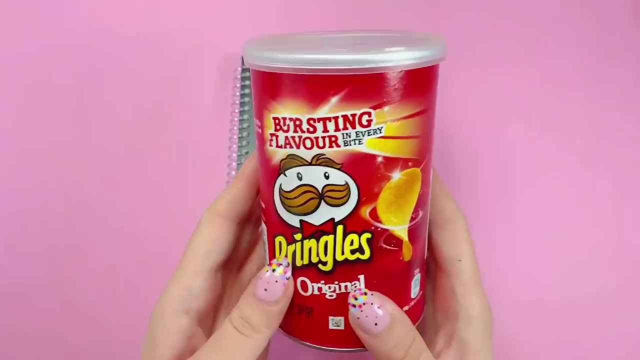 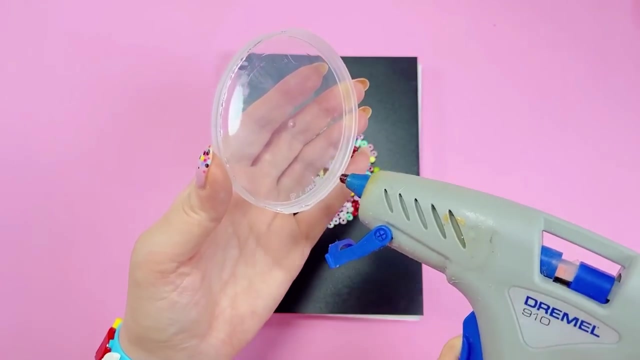 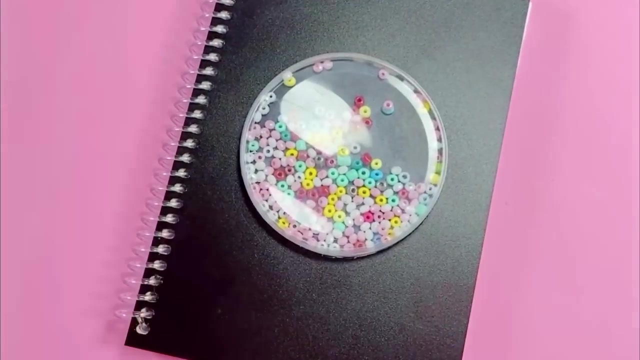 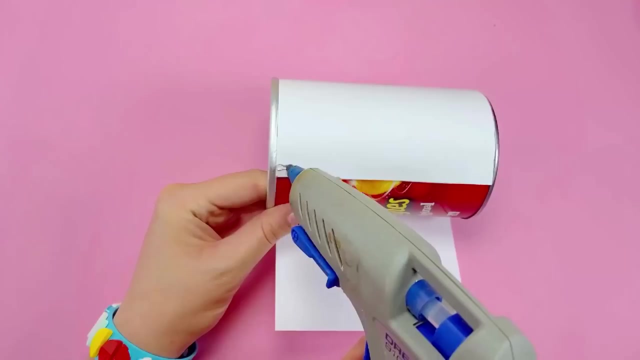 The possibilities could have happened more tonight, But no, no, we'll wait till tomorrow. Tomorrow, oh, oh. Do you think that you can call me back tomorrow? This rhythm's still swaying. I bet you think that I'm playing Hot. damn, you're making a name. 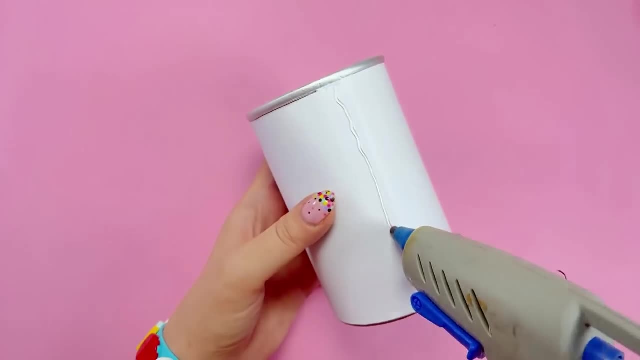 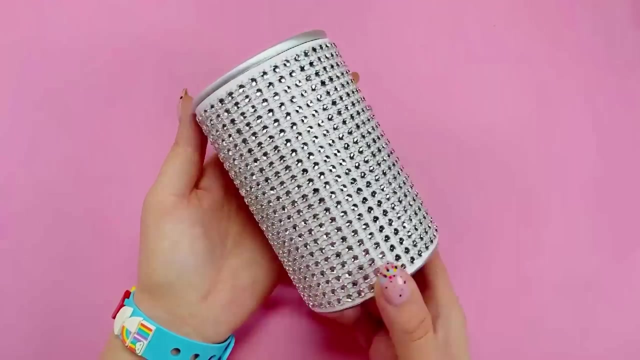 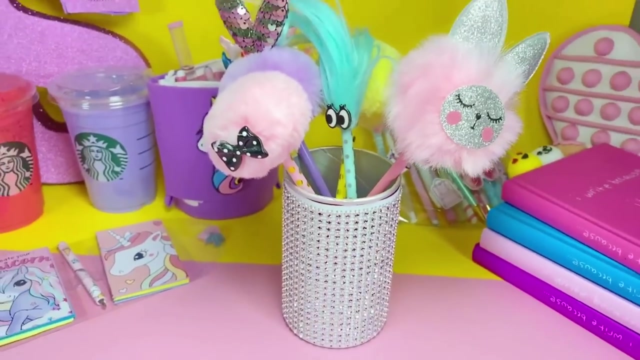 And I'm changing the game. you're gonna remember my name. You can see me moving. I'm accelerating At the speed of light. the speed of light. I can see the music moving in your veins. You know I own the night. I own the night. 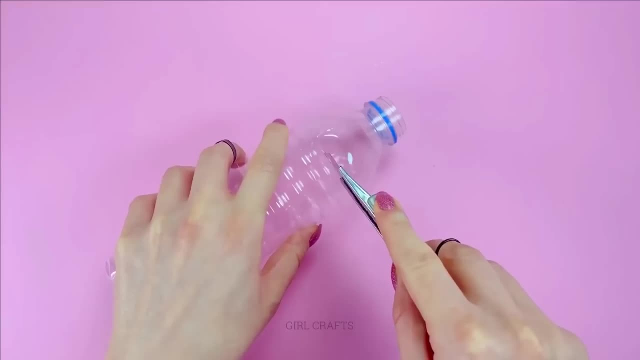 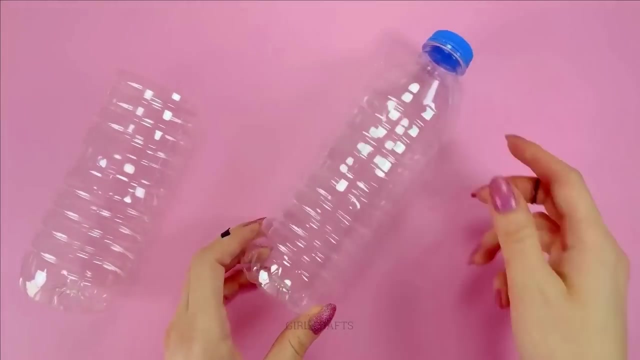 Got something to say: get out of my way. I'm here to stay and you can't stop. Get out of my way. I'm here to stay and you can't stop. Baby, you can't stop me. Got something to say? you got something to say. 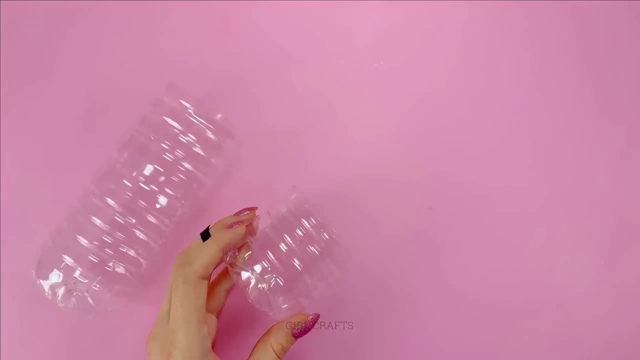 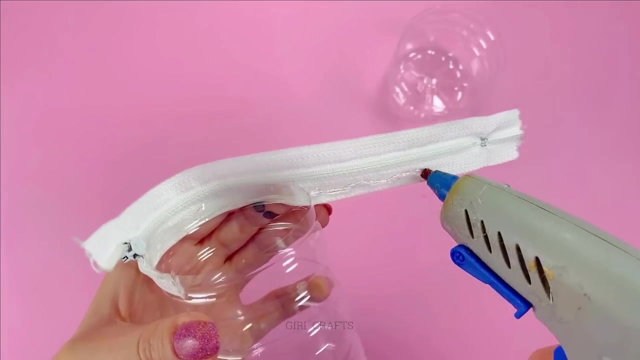 Get out of my way, just get out of my way. I'm here to stay and you can't stop me. you can't stop me, Yo. I see your mouth move, but you ain't saying nothing. What you gotta prove, I don't do the frontin'. 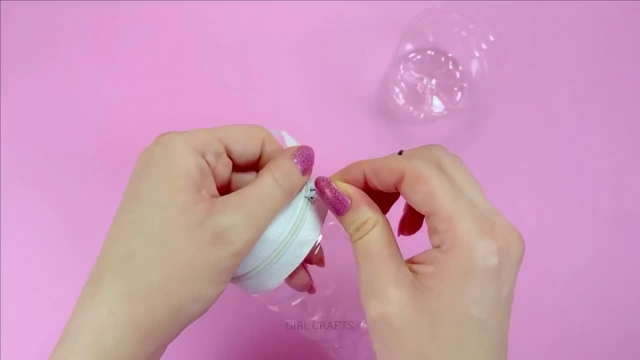 I say what I mean, mean what I say. I don't play sidestep the fake. do it in my way. I'ma call these dudes out. funny with the hate Cause your words don't make sense, like parking in the driveway. 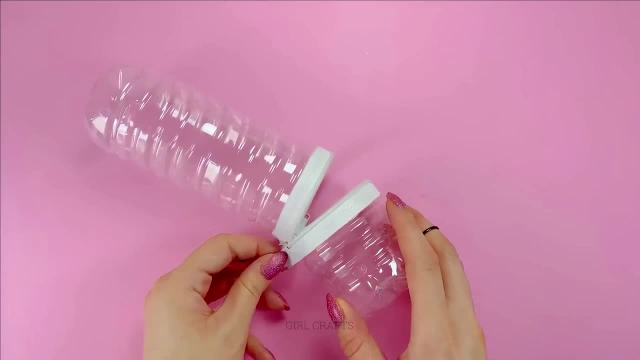 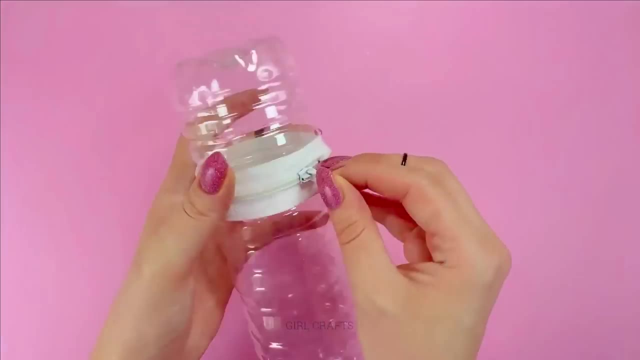 You can take the low road, I'ma take the highway. All I do is win bet that hurts to you. Baby, you can't stop me, You can't see me movin'. I'm acceleratin' Like the speed of light- the speed of light. 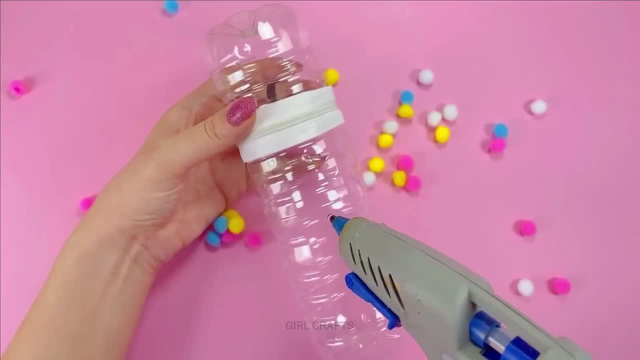 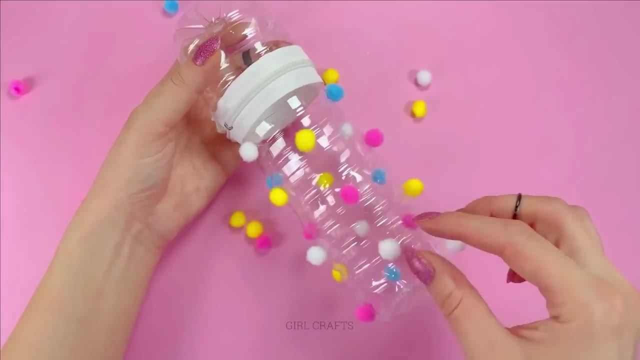 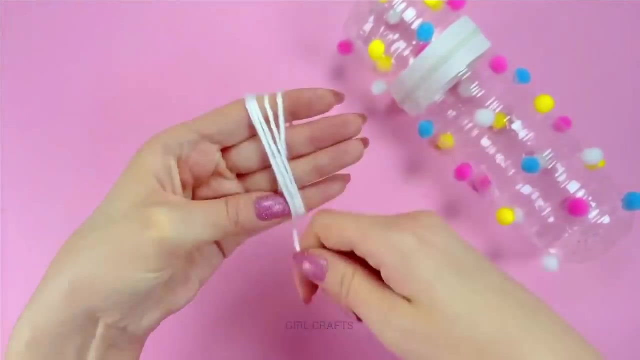 I can't see the music movin' in your veins. You know, I own the night. I own the night. Got something to say: get out of my way. I'm here to stay and you can't stop me. you can't stop me. 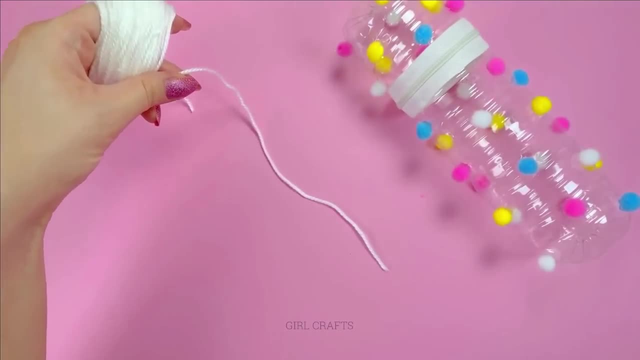 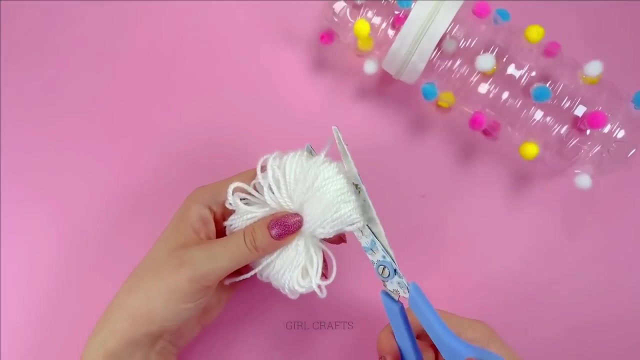 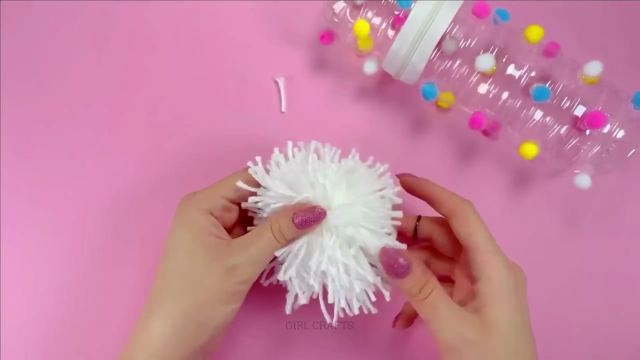 Got something to say: get out of my way. I'm here to stay and you can't stop me. you can't stop me. Hey, I can see that you don't comprehend that. I'm the best. I got my city on my back and got an S up on my chest. 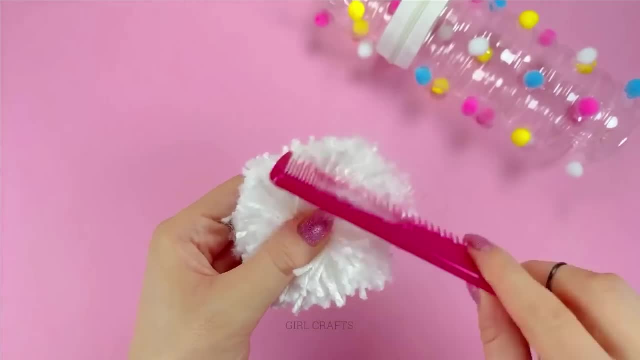 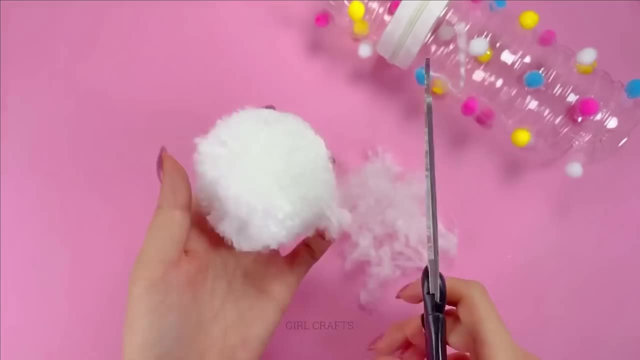 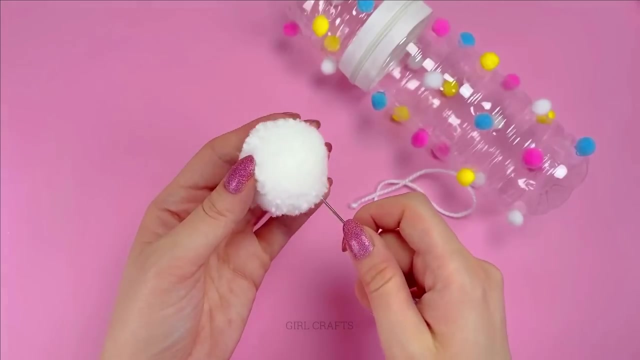 If you think you gon' come and take what I've been workin' for you wrong, I'm here to stay. this throne is mine. it's exactly where I belong. Got something to say? Get out of my way. I'm here to stay and you can't stop me. you can't stop me. 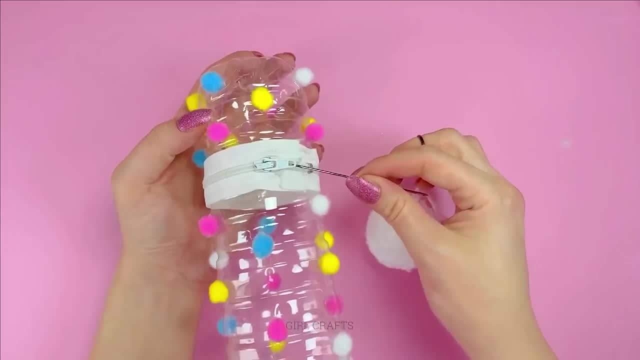 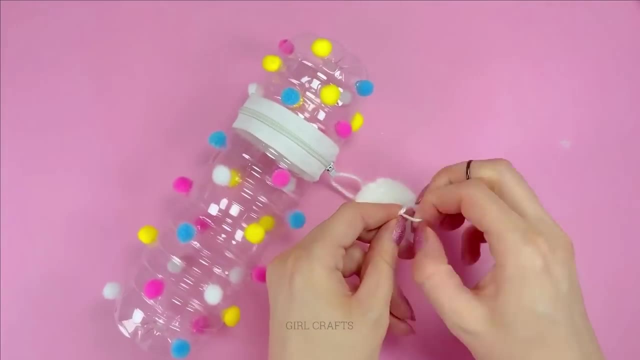 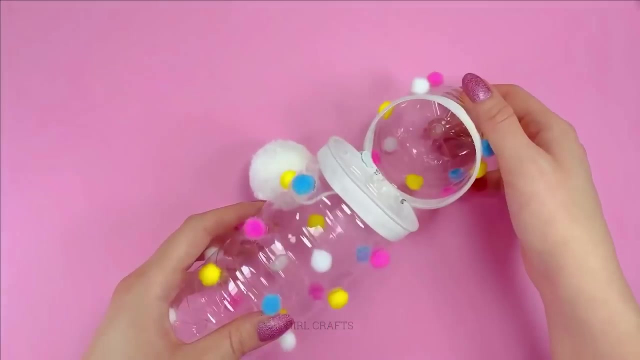 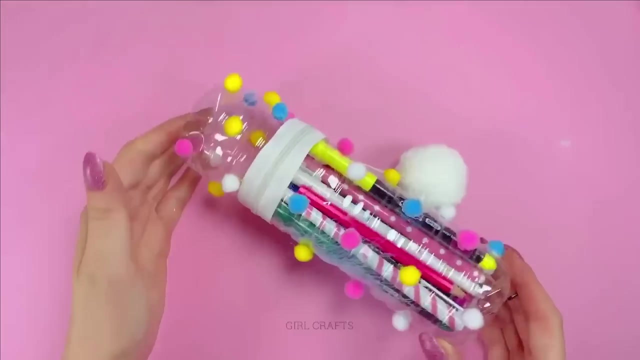 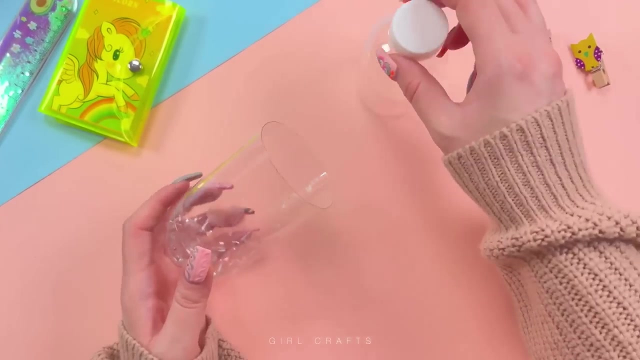 Got something to say: Get out of my way. I'm here to stay and you can't stop me. you can't stop me. Oh, I can't believe he loves me like he does. He takes my hand and flies my heart to the moon. It's what it's like when he's lovin' you. Oh, I can't believe he holds me like he does. You think that I could act my age, but it's true. I'm like a child when I'm lovin' you. Ooh, I'm like a child when I'm lovin' you. 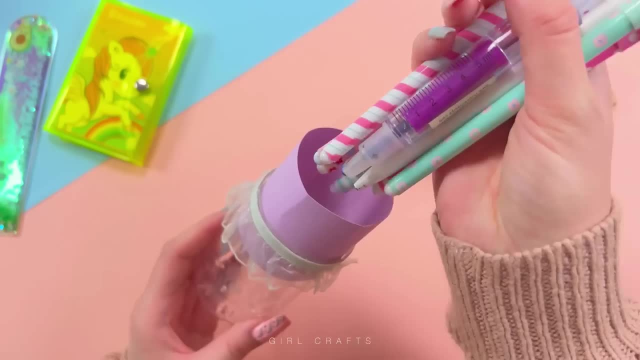 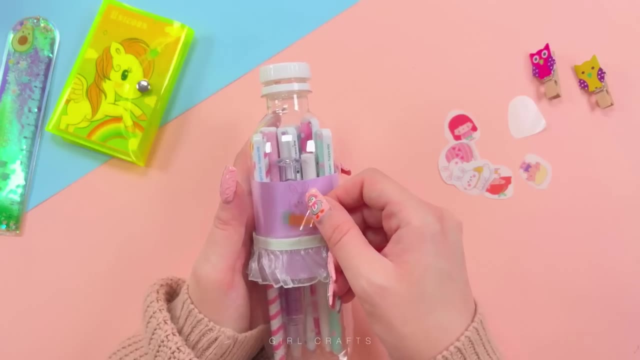 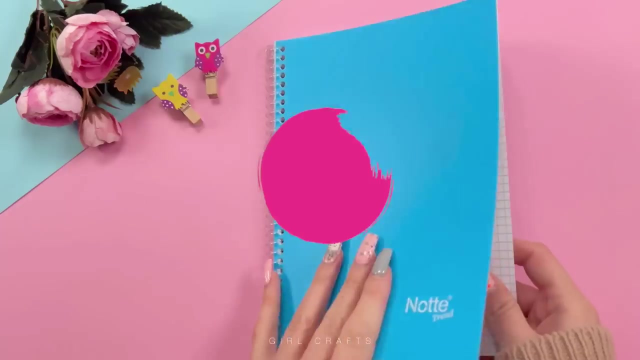 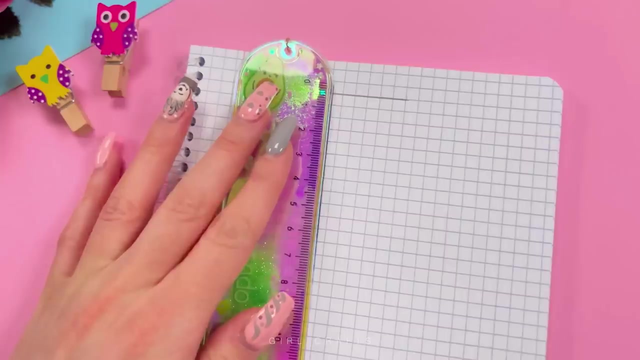 Ooh, he stole my heart. it's oh so wonderful. Oh, I gotta have him, I gotta have him. Oh, I can't imagine what I'd do without him. Oh, I gotta have him, I gotta have him. Oh, he stole my heart. it's oh so wonderful. 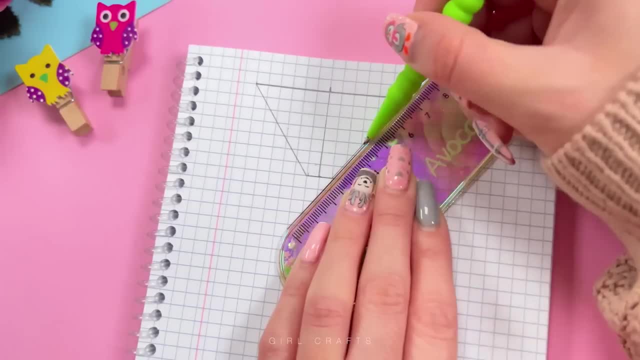 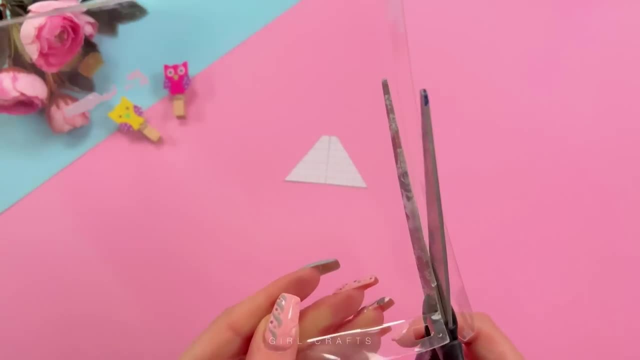 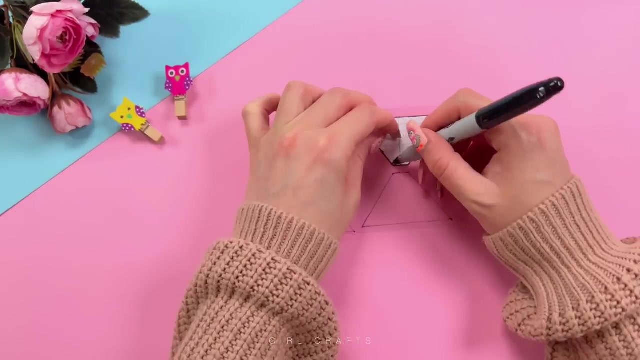 Oh, I can't believe he kissed me like he did. I could never dream of something like this. I think there's heaven in his lips. Oh, I can't believe he loves me back. I never wanna be with any other man. He takes me as I am. 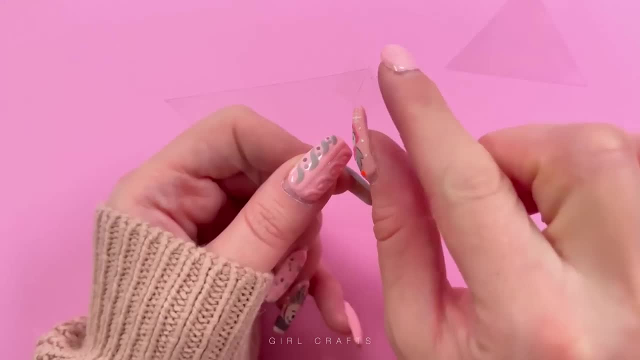 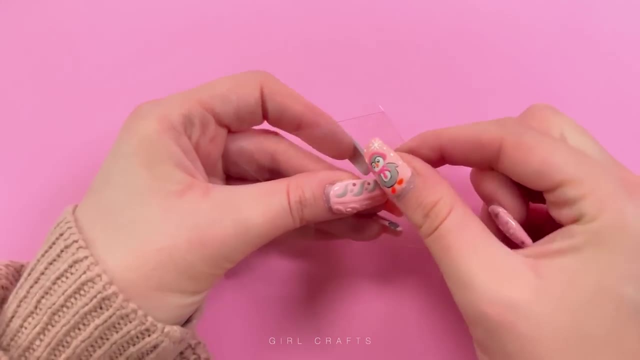 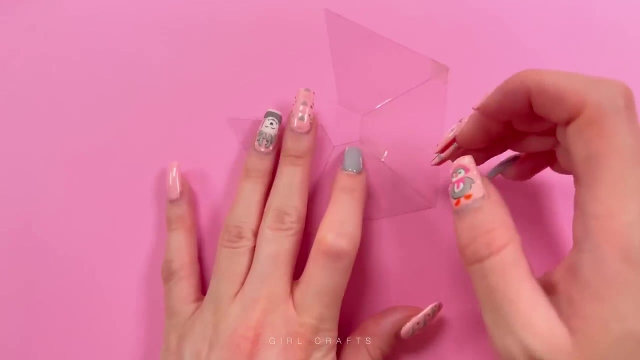 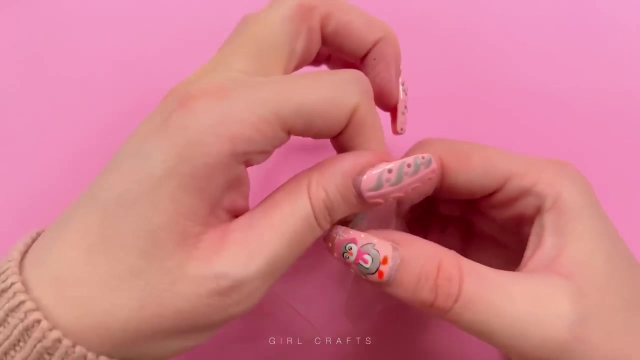 Ooh, you know, he takes me as I am. Ooh, Ooh, he stole my heart. it's oh so wonderful. Oh, I gotta have him, I gotta have him. Oh, I can't imagine what I'd do without him. Oh, I gotta have him, I gotta have him. 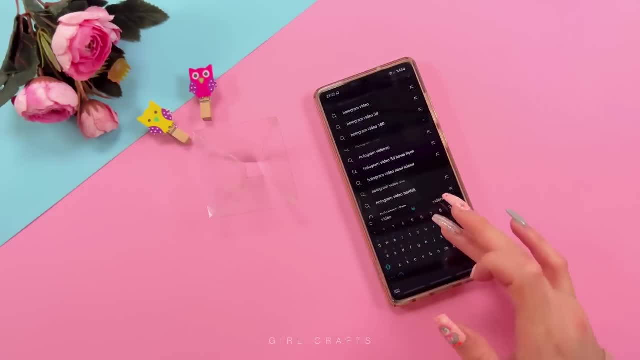 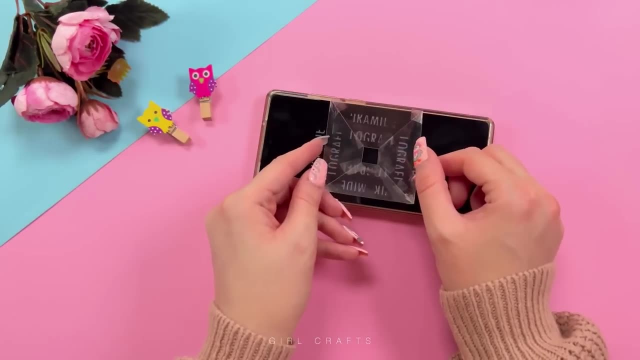 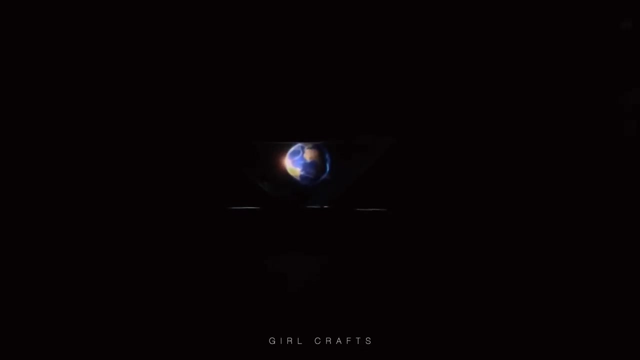 Oh, he stole my heart. it's oh so wonderful. When you're not around, I can't think. When you're not around, I can't sleep. When you're not around, I know just what I need. When you're not around, I can't think. 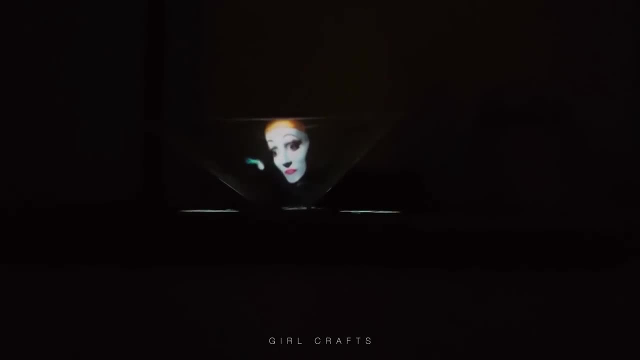 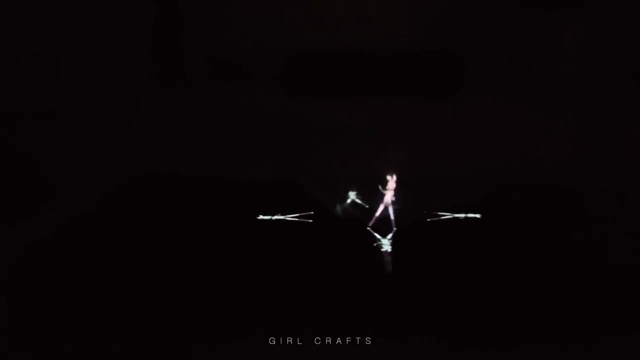 When you're not around, I can't sleep. When you're not around, I know just what I need. Oh, when you're not around, I can't think. Oh, when you're not around, I can't sleep. Oh, when you're not around, I know just what I need. 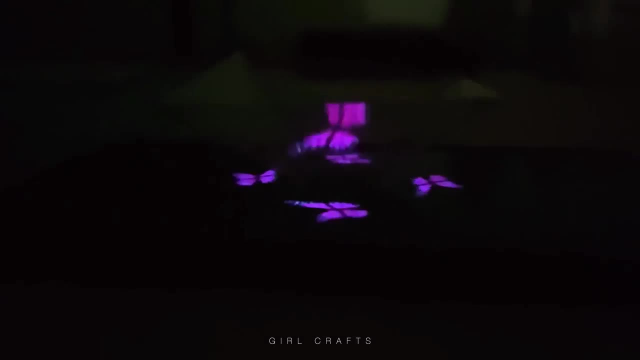 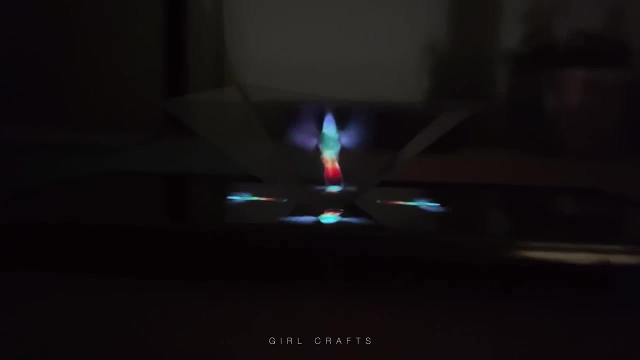 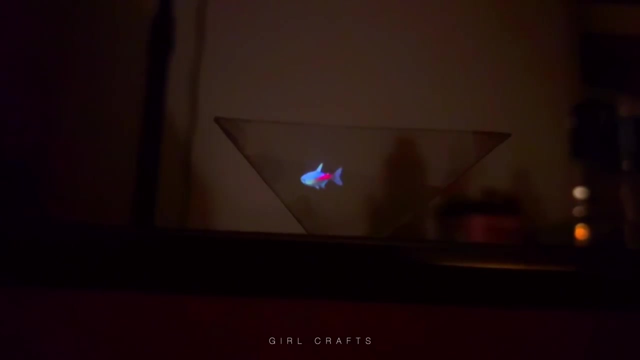 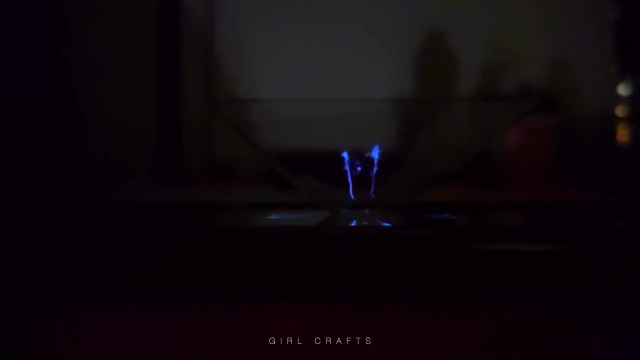 He stole my heart. it's oh so wonderful. Oh, I gotta have him, I gotta have him. Oh, I can't imagine what I'd do without him. Oh, I gotta have him, I gotta have him. Oh, I gotta have him, I gotta have him. 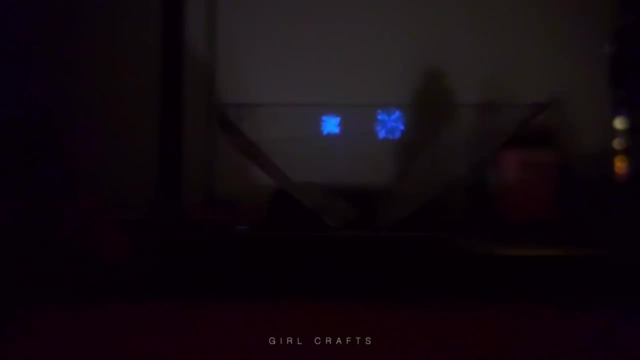 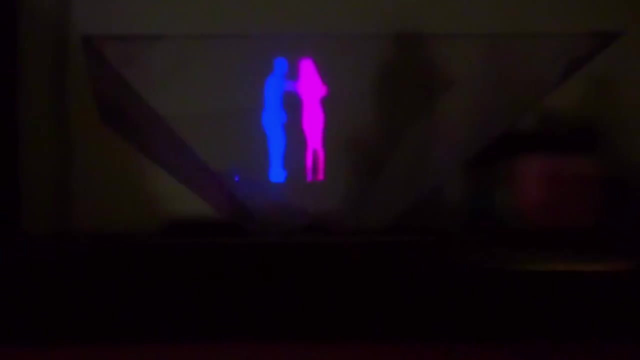 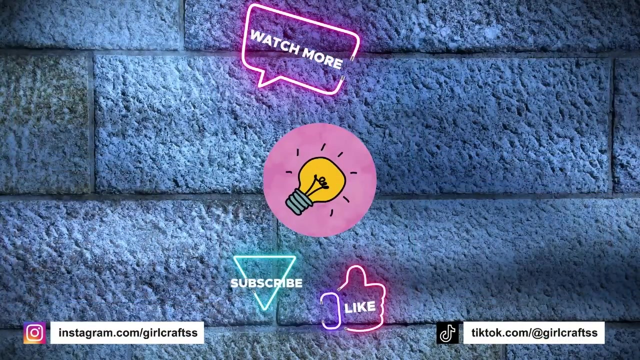 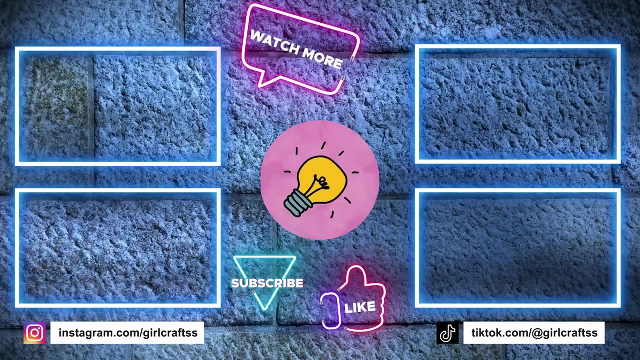 Oh, I gotta have him. I gotta have him. He stole my heart. it's oh so wonderful. I know I let love slip away And I know you're done with me, But when I see your pretty face I can barely breathe, And I know you're done with me. 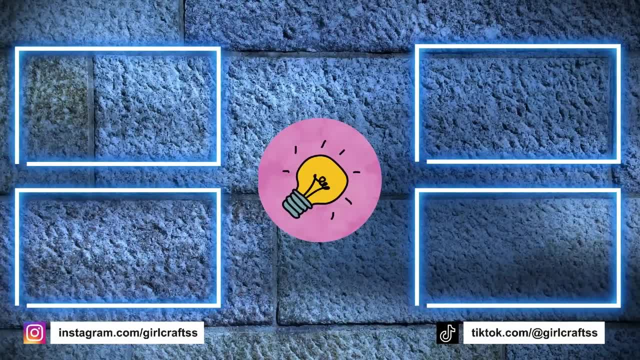 But when I see your pretty face, 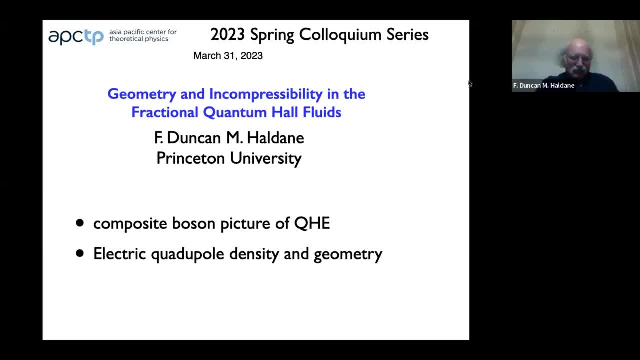 Okay, Okay. so I think it's time to start, because it's already two minutes past 10.. Okay, very good. So let me just give you a short introduction to Professor Haldane- although Professor Haldane needs no introduction in our community. And to give you a short 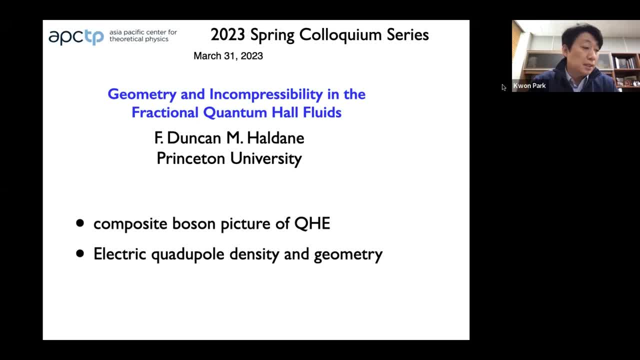 summary of his career. he has received his PhD from University of Cambridge 1978, under the supervision of P W Anderson, which reminded us that a great physicist is raised by another great physicist- And Professor Haldane became a professor in University of Southern California. 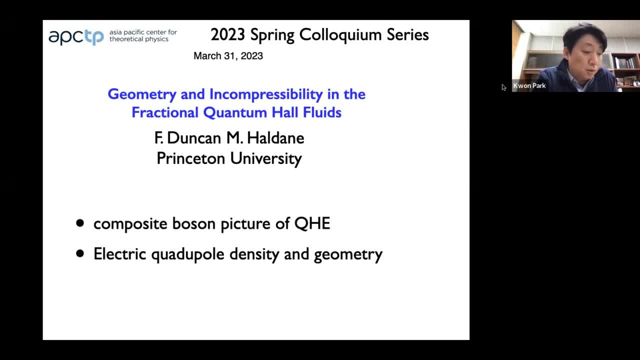 and moved to Bell Lab And again University of California, San Diego. And finally, since 1990, he has been a professor in Princeton University. He has numerous honors and awards, For example Oliver E Berkeley Contest Medal, Physics Prize in 1993 and Dirac Medal 2012.. And, of course, 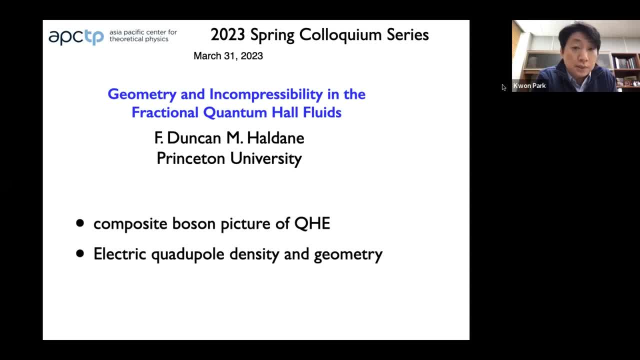 the Nobel Prize in Physics in 2016, jointly with the University of California San Diego and the University of California San Diego. And, of course, the Nobel Prize in Physics in 2016, jointly with the University of California ine.